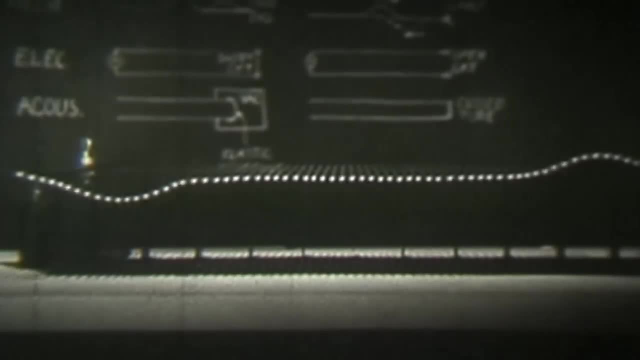 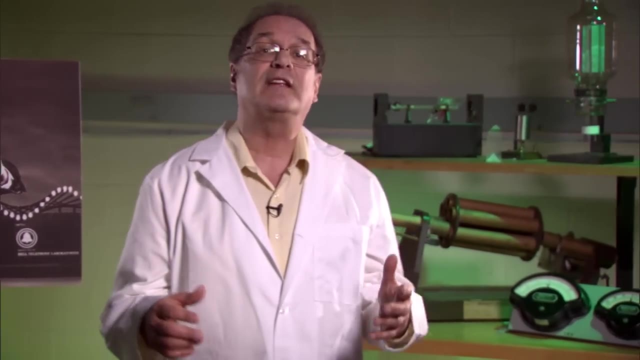 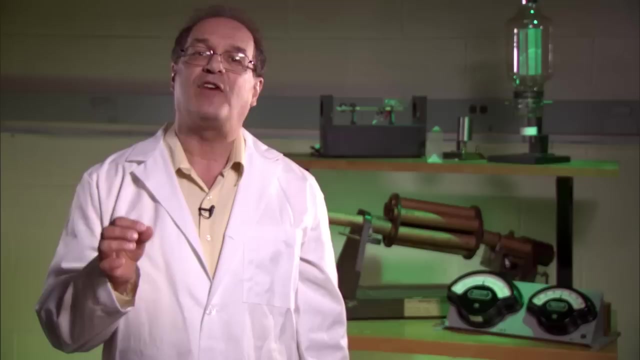 wave motion concepts across disciplines from the electrical to the physical, to the spectral. The machine made its public debut in this film and was released along with the companion book. It was part of a general effort on the part of AT&T's Bell Labs to provide 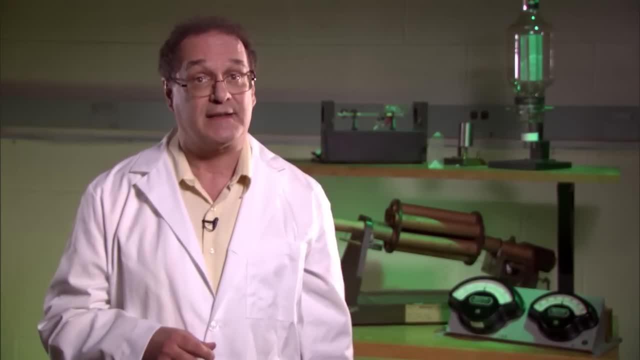 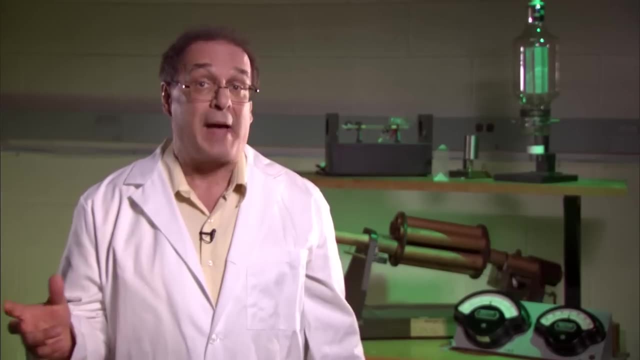 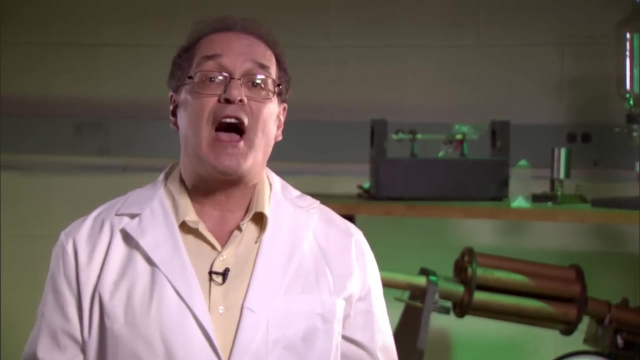 novel educational tools for the next generation of scientists. Now it's a staple in physics classes around the world. You can still buy one newly manufactured, though it would be worth the money. Besides being an inventive engineer, Shive was also a gifted lecturer. 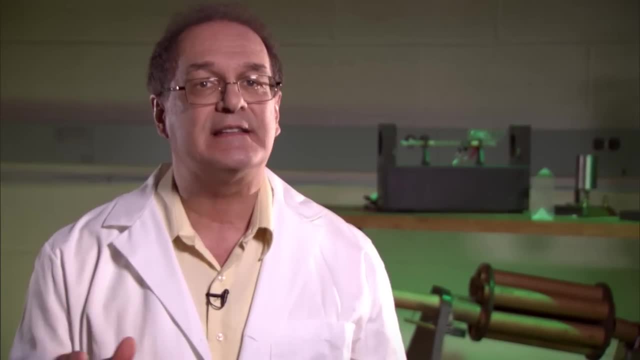 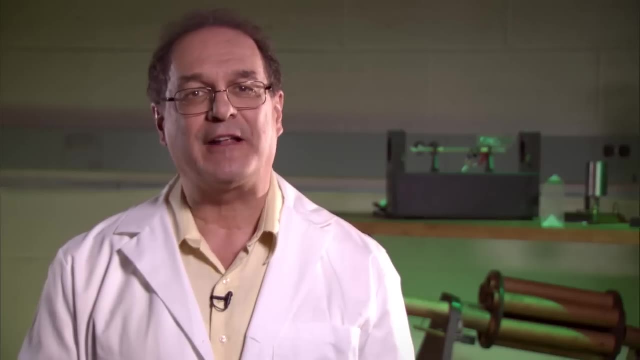 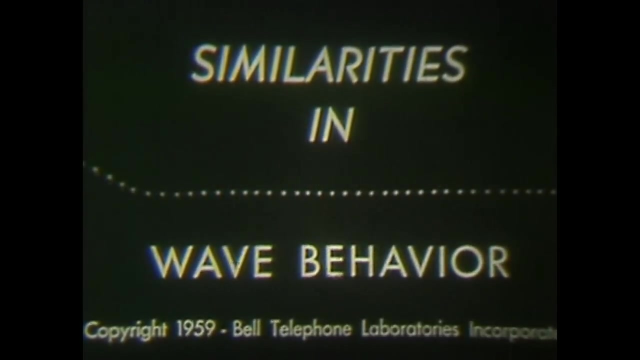 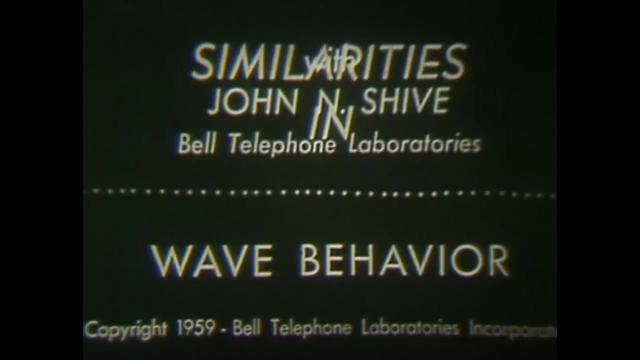 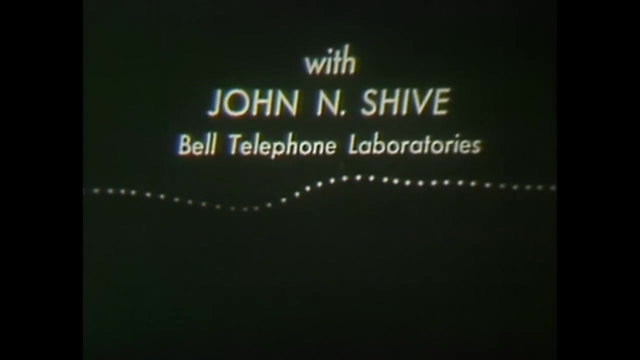 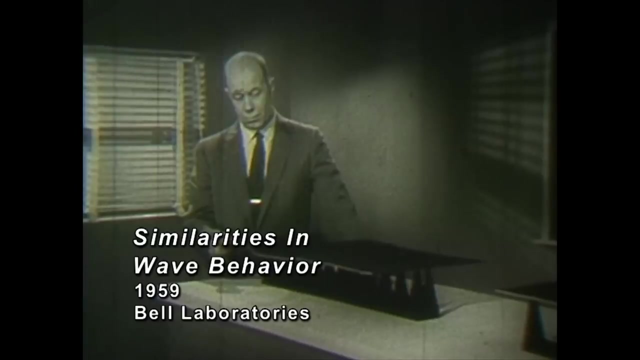 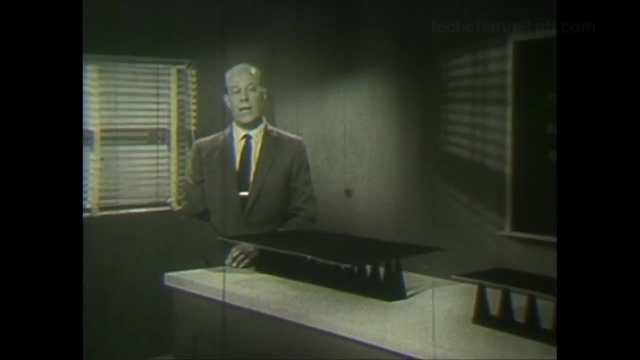 and he deftly projects his love of physics in this 1959 film Straight from AT&T Archives and History Center. here's Similarities of Waved Behavior. People who study waves extensively in the various fields of physics and engineering are impressed by the similarities which exist in the behavior of waves in various mechanical 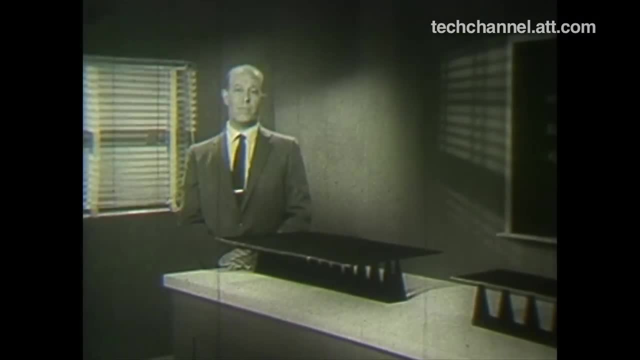 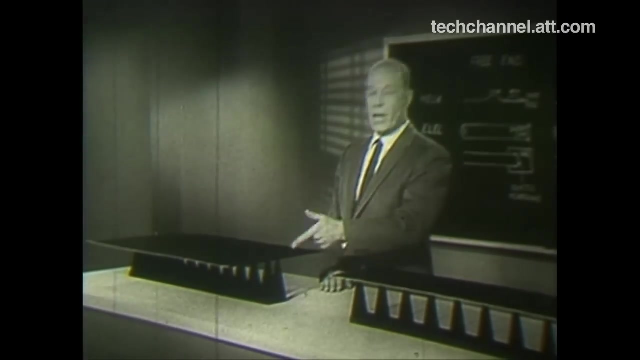 and electrical systems, The development of waves in the various fields of physics and engineering: electrical, acoustical and optical wave systems. These similarities are due, of course, to the basic fact that waves of all kinds behave fundamentally alike. These two rib-like structures are mechanical wave demonstration machines. 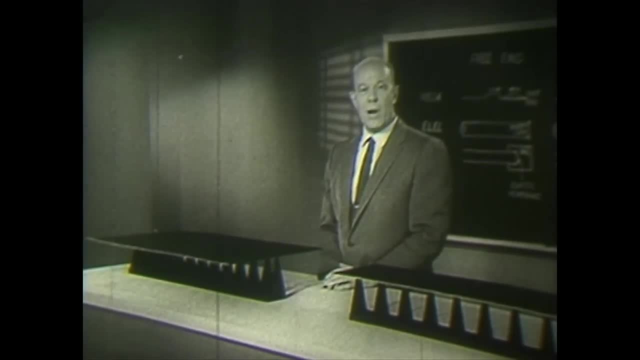 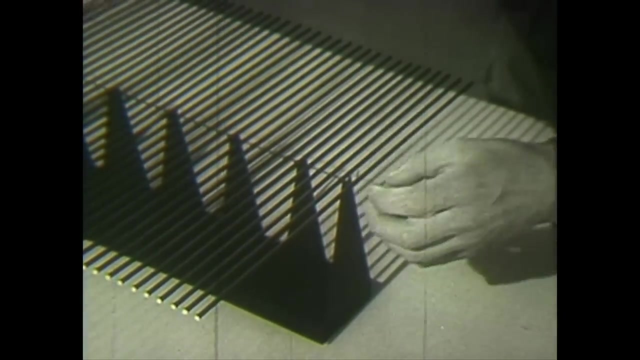 With them, I can show you many of the various wave properties which you may have studied, experimentally or theoretically perhaps, without ever having actually seen what the waves themselves are doing. The waves which travel on this machine are really waves of twist or torsion which propagate. 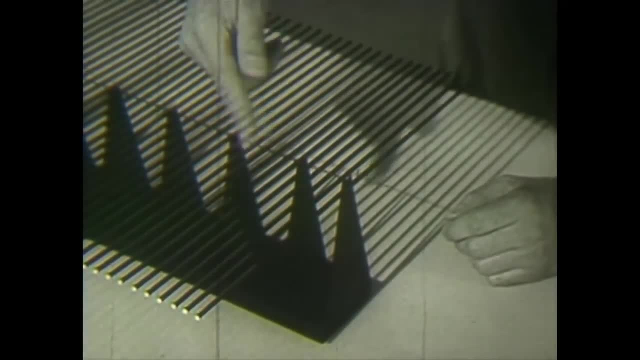 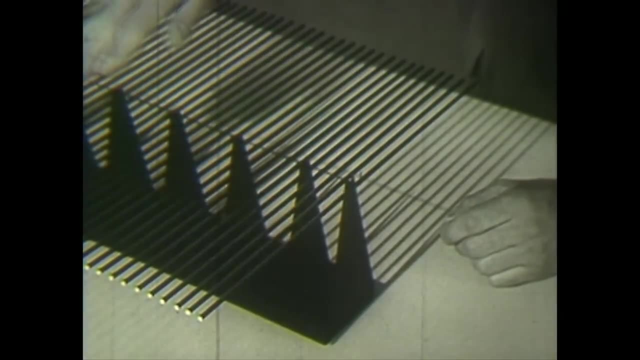 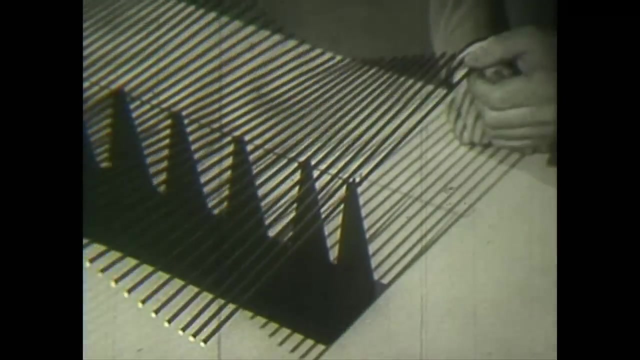 along this central wire. Attached to the central wire are these cross arms which translate the torsional motion of the central wire to the up and down transverse motion of the ends of the cross arms which you see, The entire structure is supported in a set of bearings which permit the 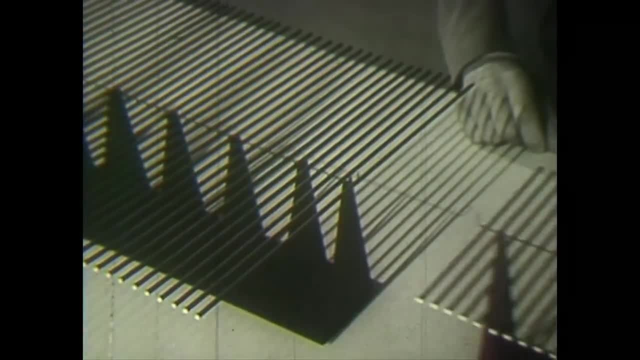 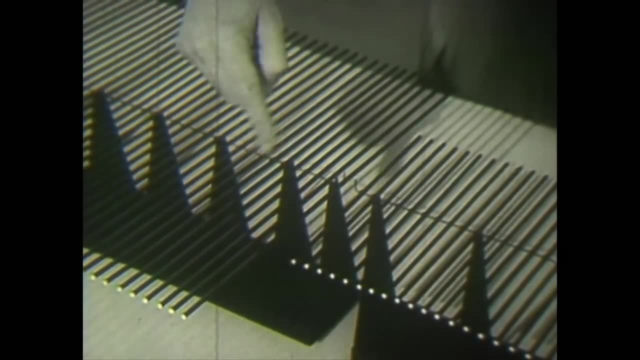 central wire to move in and out of the cross arms. The entire structure is supported in a set of bearings which permit the central wire to twist freely. This second wave machine is built similarly to the first. It has cross arms which are considerably shorter than those on the first machine. 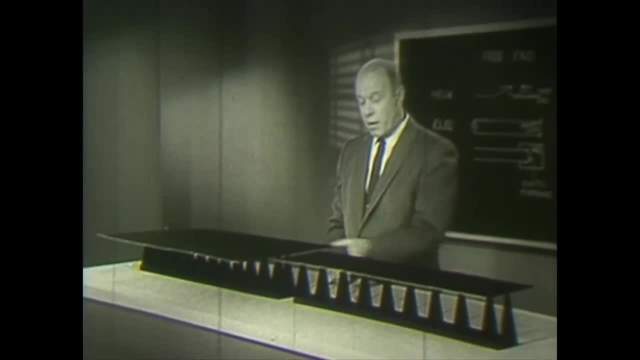 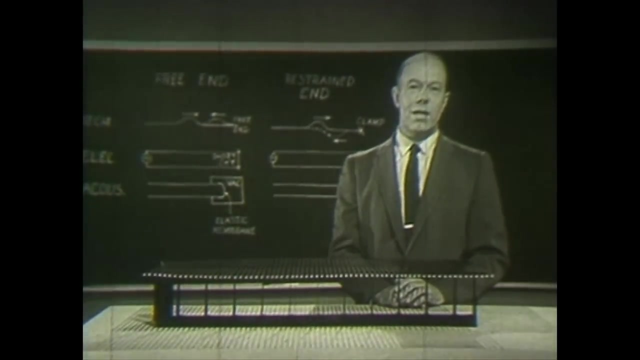 and, as a consequence, the speed of a wave along the second machine is about three times faster than the speed of a wave along this machine. You'll see later on why I have these two machines. First, I want to show you the two different ways in which waves may be totally different. 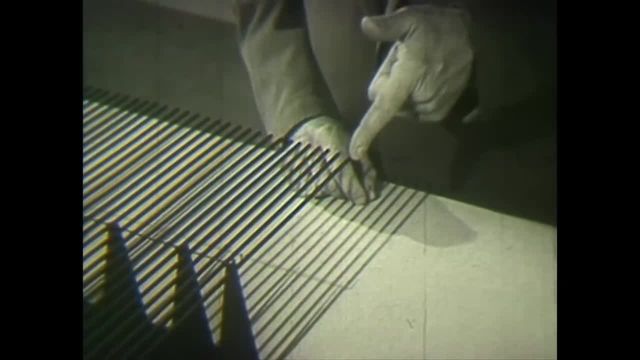 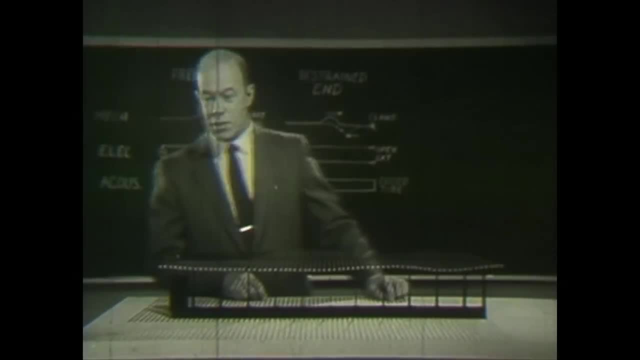 First, I want to show you the two different ways in which waves may be totally reflected. Observe that right now this machine has a free end, That is, this last cross arm is perfectly free to move without restraint. If I start a wave at this end of the machine, that wave travels down to the far end is reflected. 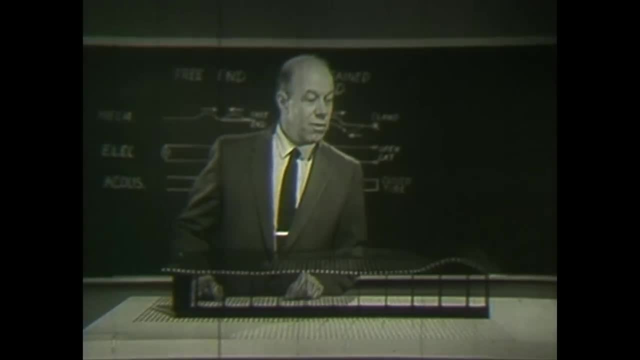 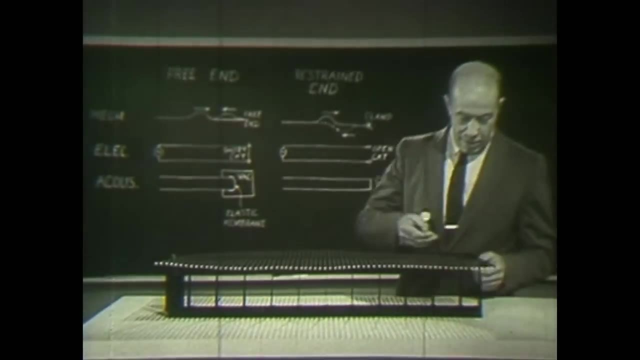 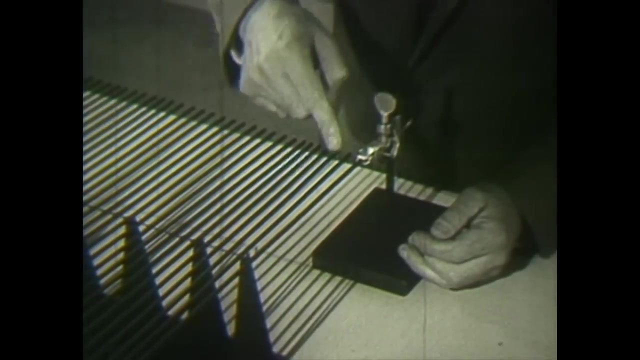 there and returns as a reflected replica of its original self. But now let me terminate this machine in a different way. I'll clamp this last cross arm to a heavy stand so that a wave arriving here can't produce any displacement of the cross arm. 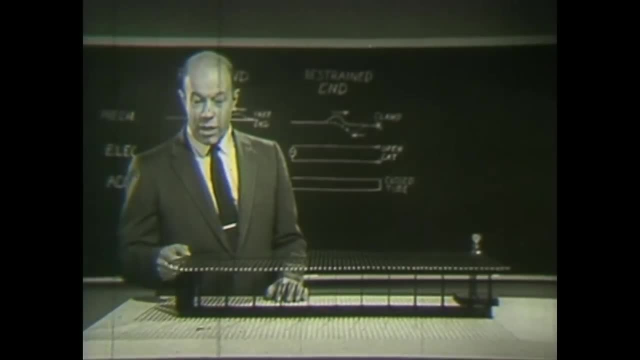 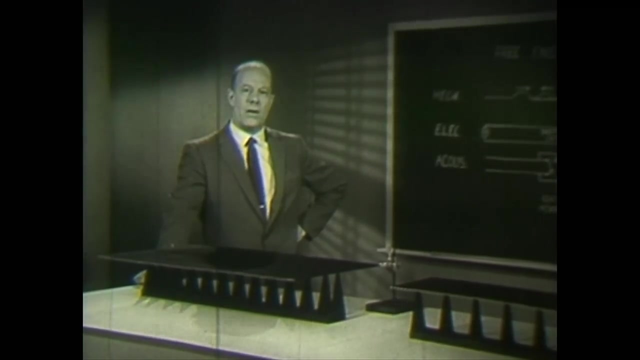 This time, you see, the wave is reflected upside down. The reflection is still total, as it was before, but the wave is inverted upon reflection. In a mechanical wave system, then there are two ways in which the total reflection of waves may take place: Right side. 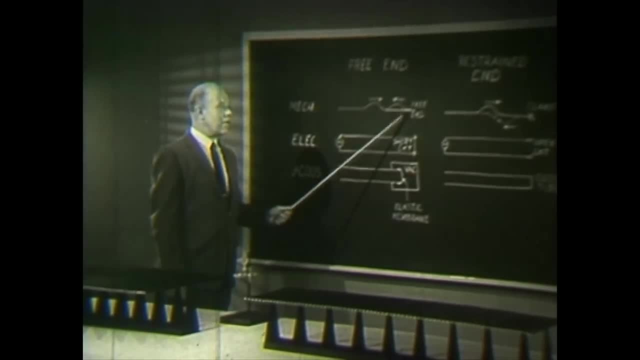 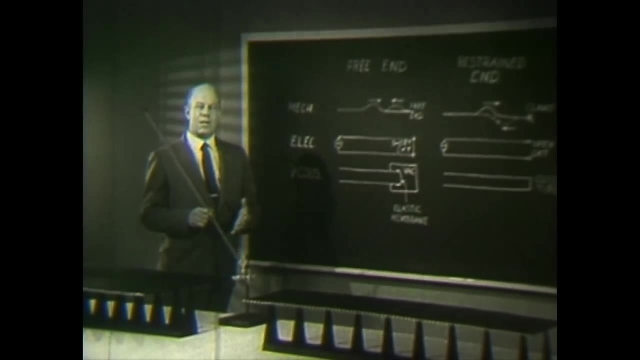 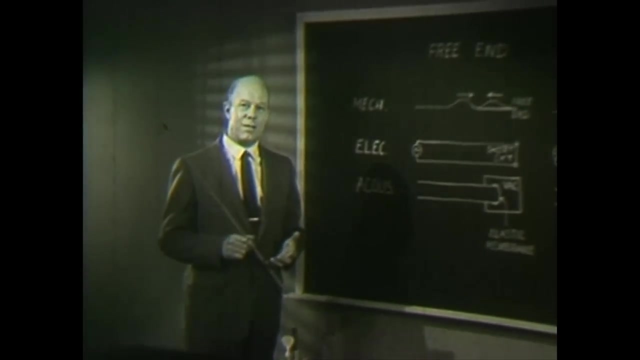 up if the reflecting end of the medium is completely free, and upside down if the reflecting end is completely restrained. Now, if nature has any consistency- and we like to think she does- this alternative reflection possibility should exist for waves of all kinds and these other drawings here. 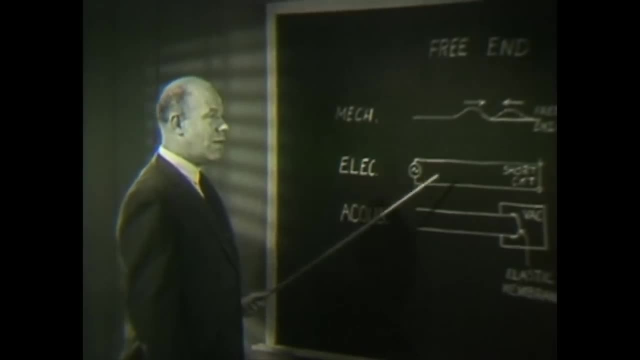 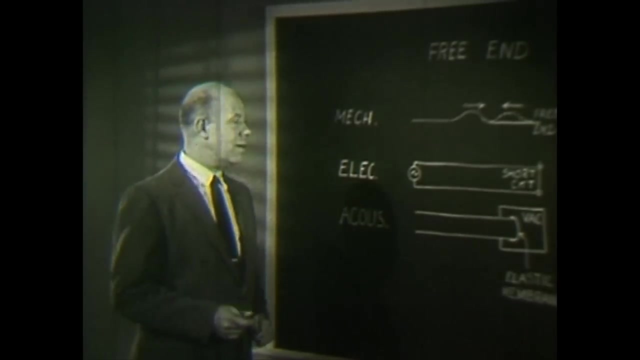 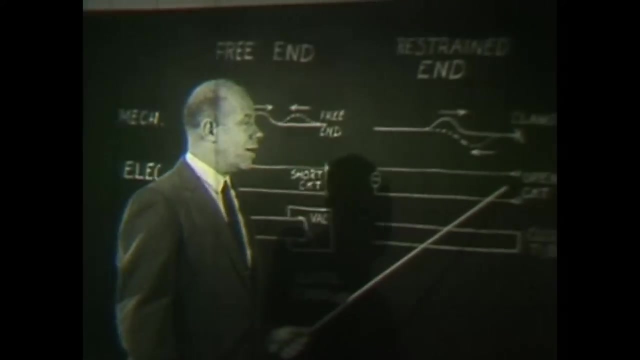 show that indeed it does. Take the case of an electrical transmission line, for example. You know that there are two ways in which electrical waves can be reflected, depending on whether the far end of the transmission line is terminated by a short circuit or by an open circuit. 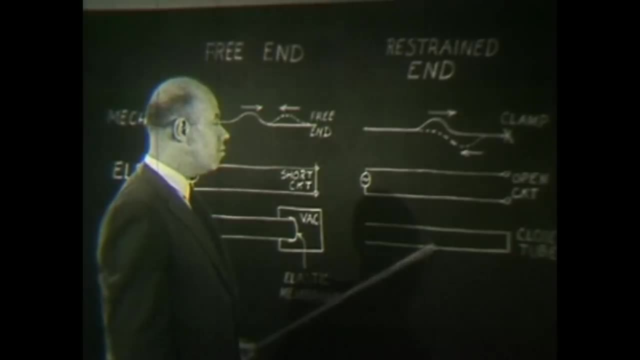 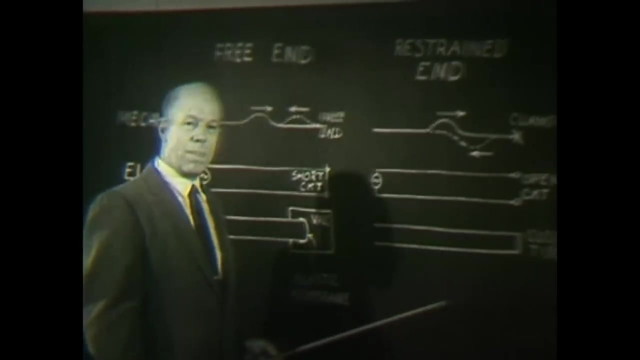 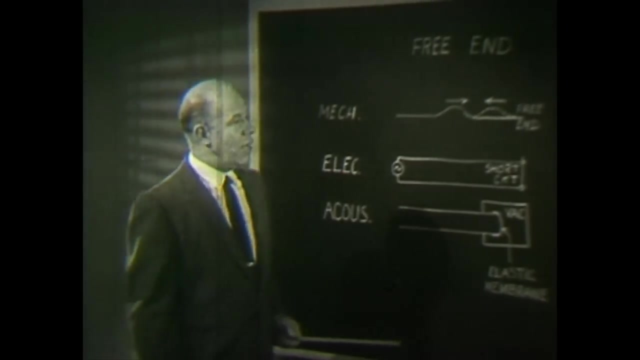 And similarly in the case of waves traveling down an acoustic tube. there are two different reflection possibilities, depending on whether the end of the tube is closed by a rigid termination or by the acoustic analog of a free end. Note that in the mechanical situation, a clamp is a constraint preventing the displacement of the end of the wave medium. 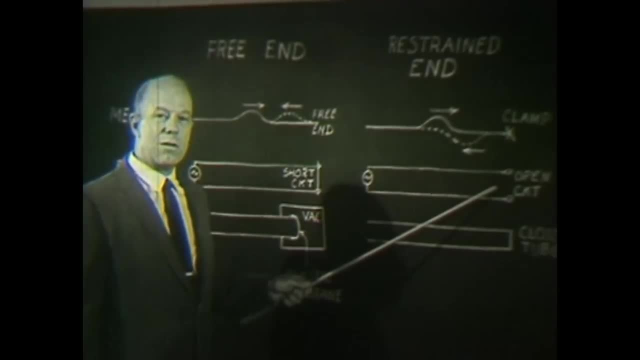 The electrical analog of this state of affairs is an open circuit termination on the end of a transmission line preventing the flow of current at such a termination, And the acoustic analog is a rigid closure at the end of an acoustic tube preventing the longitudinal vibration of the air. 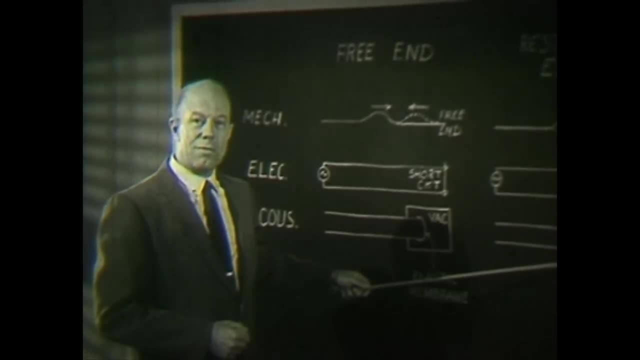 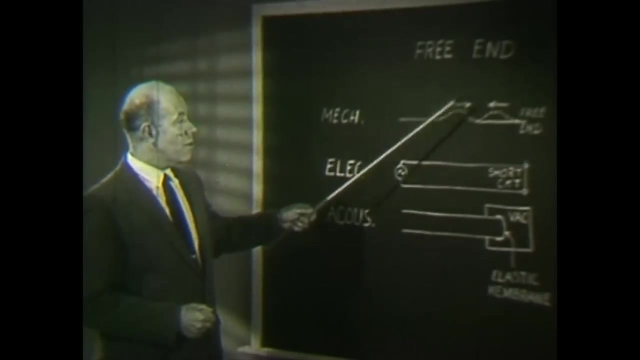 In a case of a wave medium, the clamp is a constraint preventing the displacement of the end of the wave medium. In all of these cases, the reflected waves come back upside down. And in all of these other cases, conversely, which are analogous to the case of the free end of a reflecting wave medium, 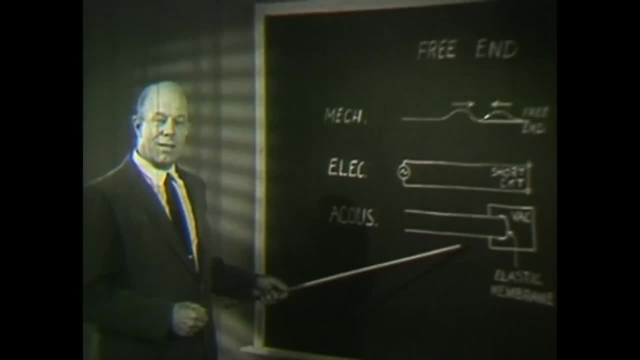 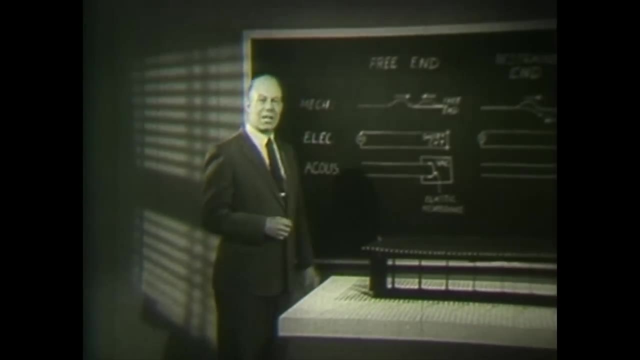 the reflected waves come back right side up. You see, nature really is consistent. Well, now let's have a look at some of the other things we can do with our wave machines. One of the most important topics in the general development of the natural world is the reflection of the wave. 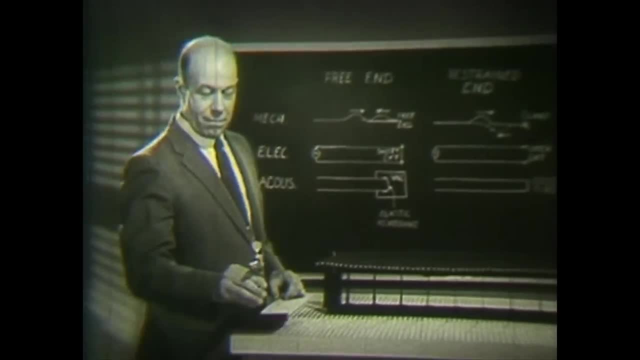 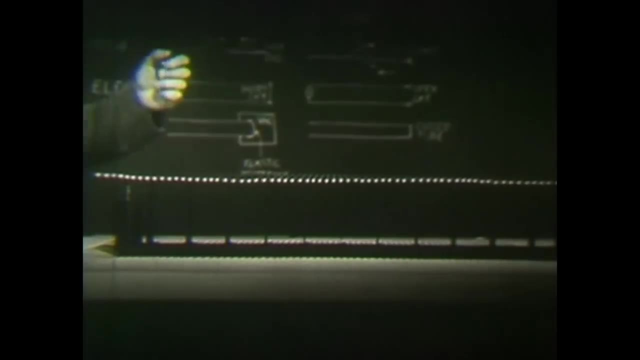 development of wave behavior is the principle of superposition. When two waves traveling in opposite directions on the same medium, as you see here, in slow motion, pass through each other, the instantaneous amplitude of the resultant wave is the algebraic sum of the amplitudes. 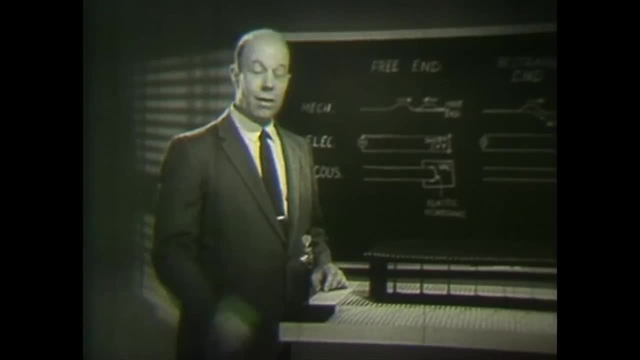 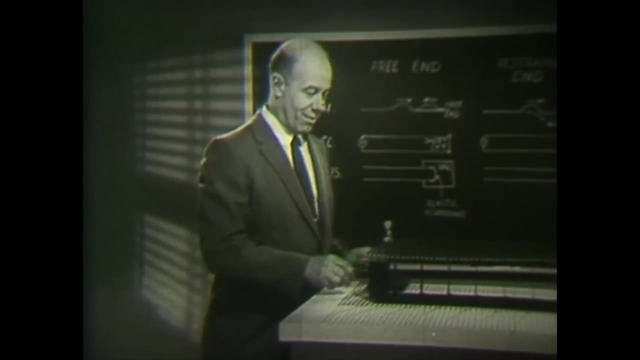 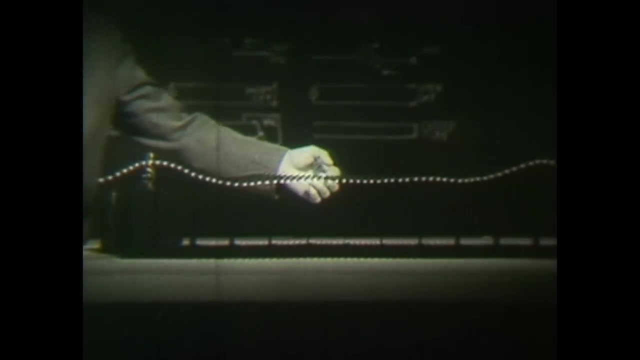 of the two constituent waves. This principle of superposition is equally valid when one of the two waves is positive and the other one is negative. Observe that in this case, at the instant of exact coincidence, there is a momentary cancellation of the amplitude. 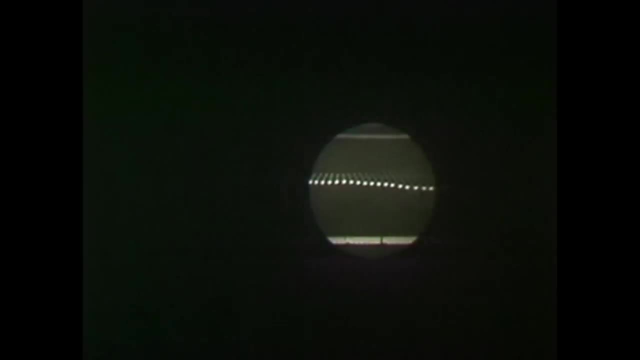 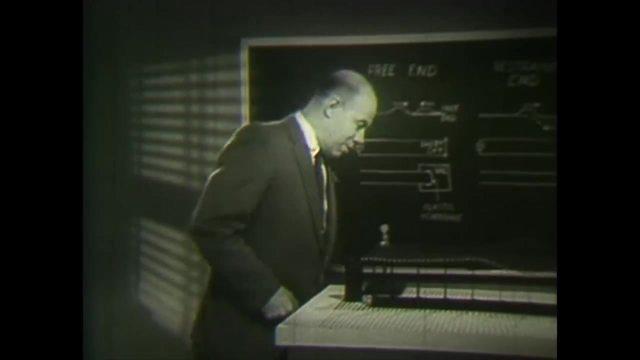 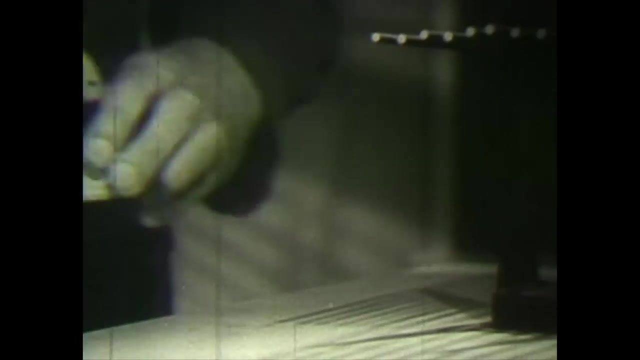 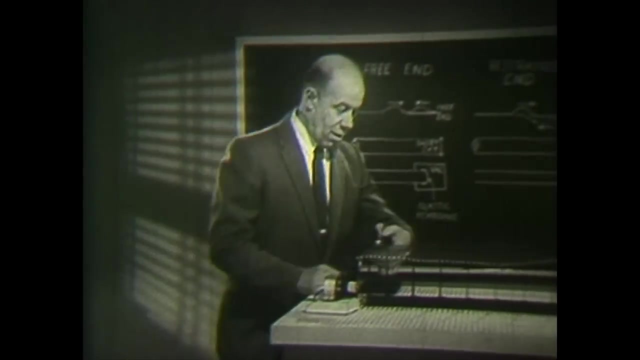 and the medium appears to be undisturbed. Now let's have a look at the superposition behavior of continuous trains of periodic waves. With this small motor and crank I can generate such a train of waves at this end of the machine and reflect them back upon themselves at this end. 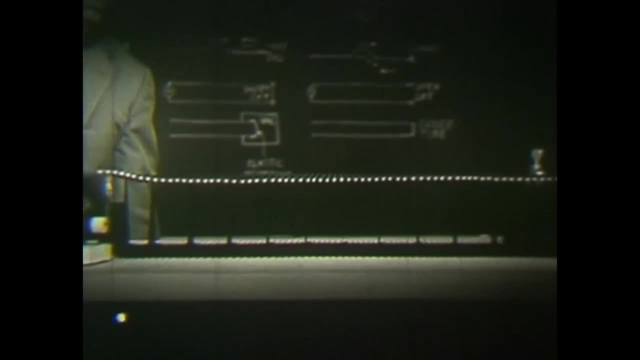 All right, in slow motion. now here come the waves. After reflection, the waves traveled back up the machine, superposing on the oncoming waves which they meet to produce patterns of built up amplitude at some places and complete cancellation at others. The pattern that you see on this machine appears to be standing still. 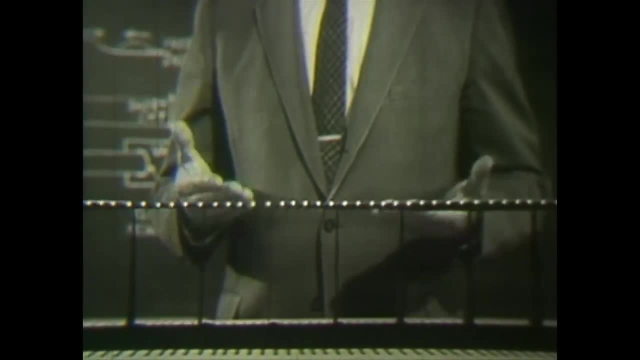 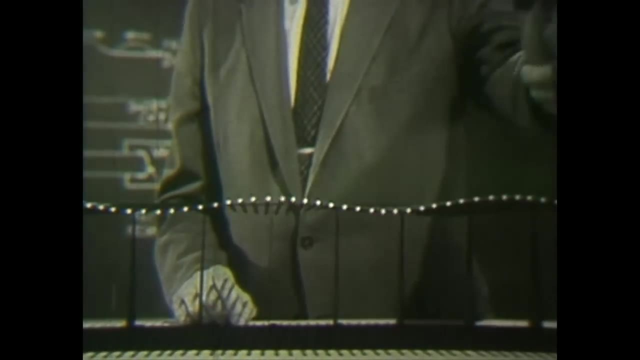 doesn't it? The various portions of the medium simply bob up and down in place without giving you the impression of motion in either direction along the machine. Let me just repeat this one time of motion in either direction along the machine. Observe that in this pattern. 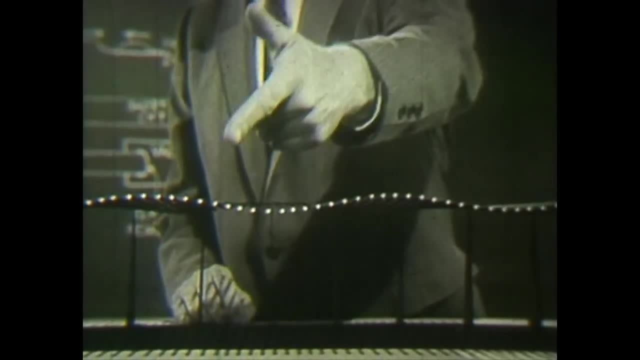 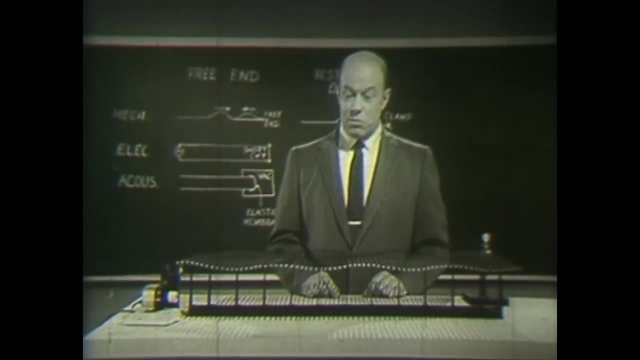 there are places where the medium appears to be standing completely still all the time. These dead spots, or nodes, are exactly half a wavelength apart. Now, I'm sure that you've all seen behavior of this kind before. For example, a vibrating string always vibrates naturally in one or more segments. 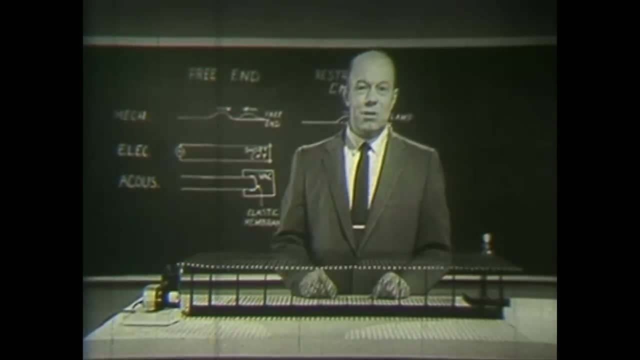 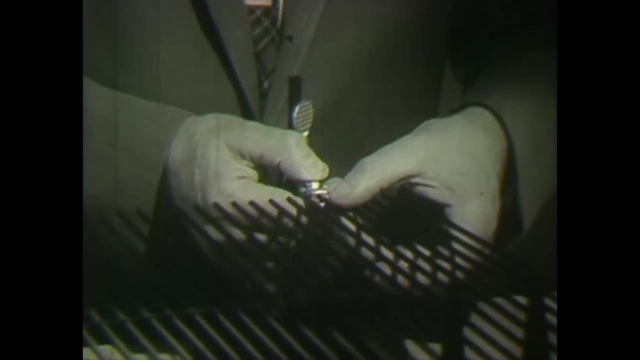 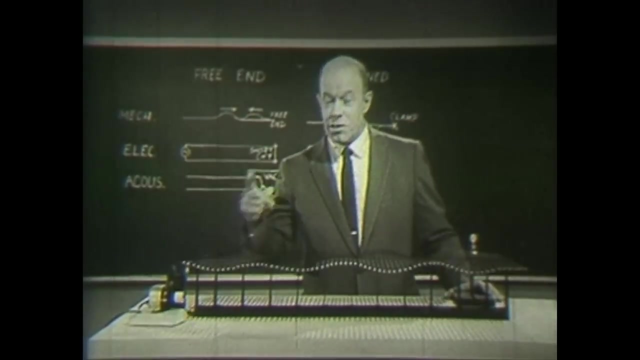 separated by such nodes. Now let me show you something else. Suppose I simply move this reflector a short distance up the line toward the generator, just far enough so that the travel time of a wave down and back is an exact multiple of the wave period. Under these conditions, the new waves which are continually 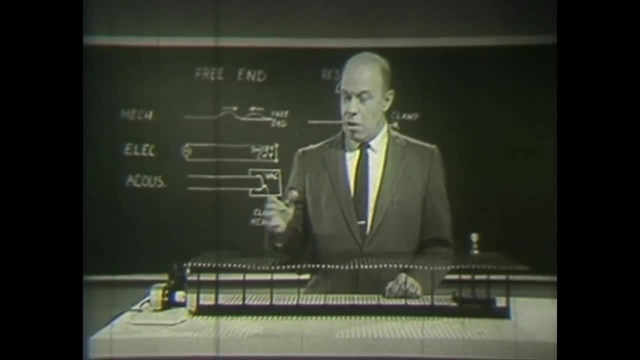 being sent out by the generator superpose upon the previously emitted and multiply-referenced waves. The new waves are then automatically reflected waves in just the right phase to build up the amplitude to an abnormally large value. new crest on previous crest, and so on. 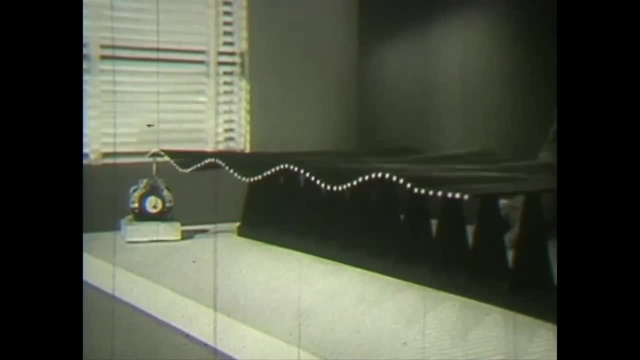 The system thereupon becomes resonant and the amplitude builds up to the noticeably larger value that you see here. Under these conditions, the new energy which is being fed into the system at each cycle is exactly equal to the energy which is being dissipated per cycle through friction. at this new 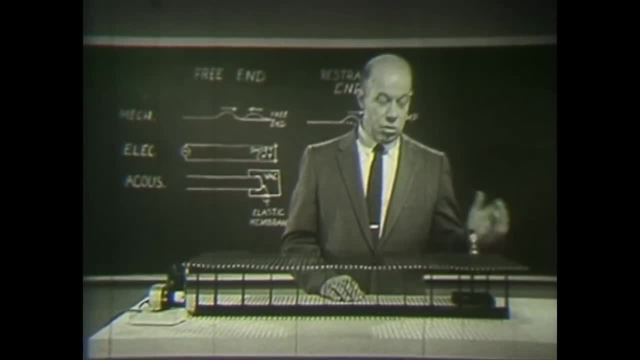 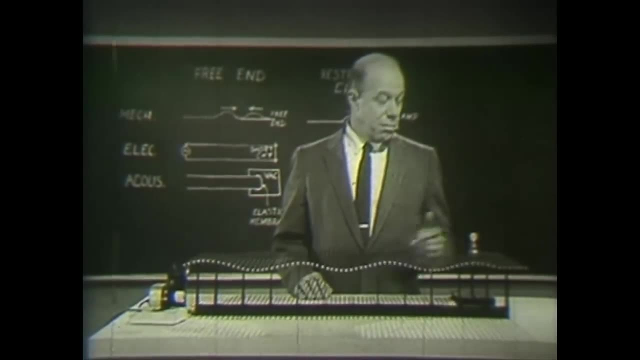 amplitude which I made in the length of the machine to produce this resonant condition is called tuning. I could just as well have produced resonance by leaving the line at its original length and tuning the frequency of the generator instead, And I can destroy the resonant pattern that I have here by 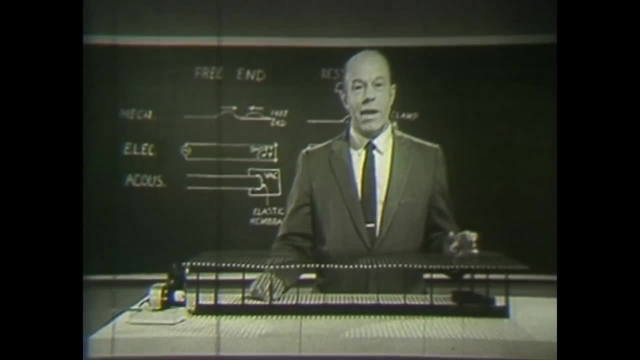 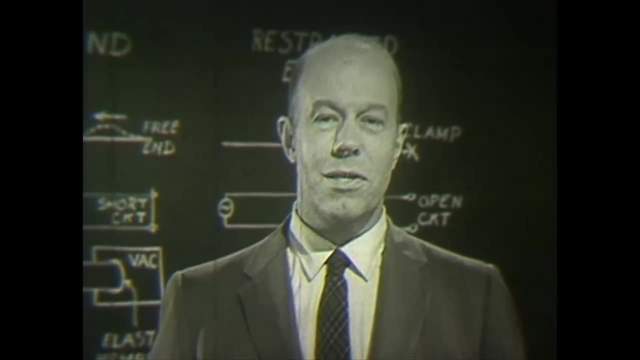 changing the value of either of these parameters a little bit in either direction. Another way of looking upon a resonant system is to regard it as a reservoir for energy. Thus, the escape wheel of a watch, a child's swing, a sounding organ pipe, the resonant circuit of an electrical radio transmitter are 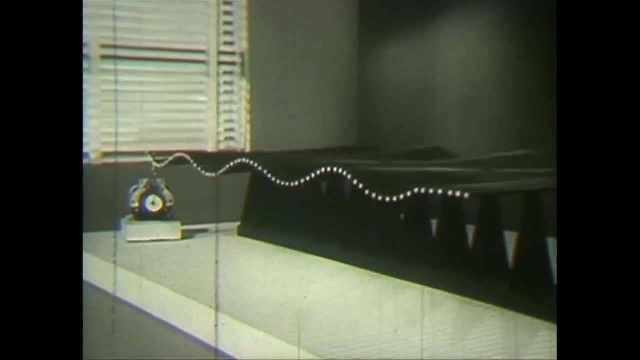 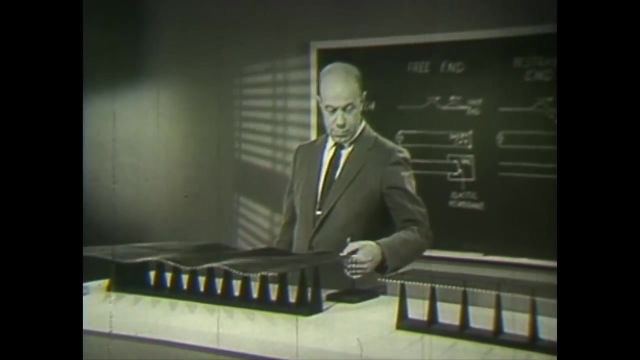 all examples of resonant systems. They exhibit abnormally large amplitudes of oscillation and they possess relatively large contents of energy which have been built up by superposition over many previous cycles. Now, from here I want to go on to the subject of the impedance of the wave. 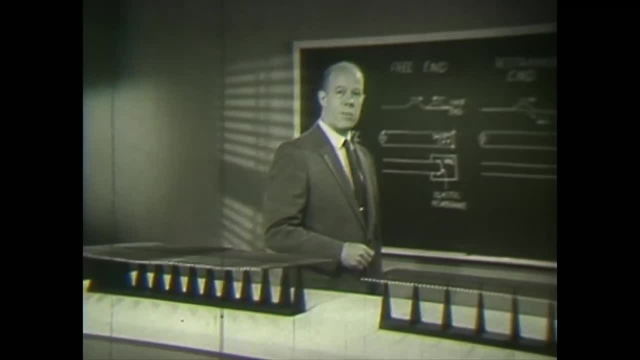 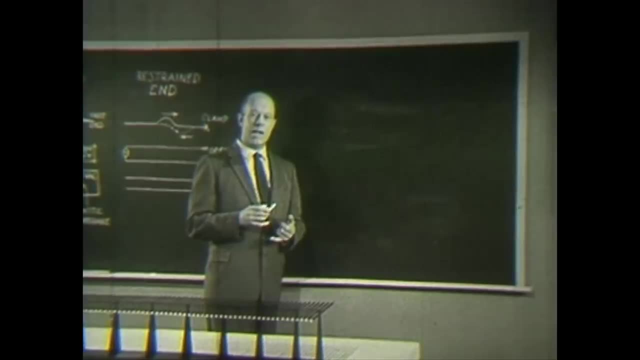 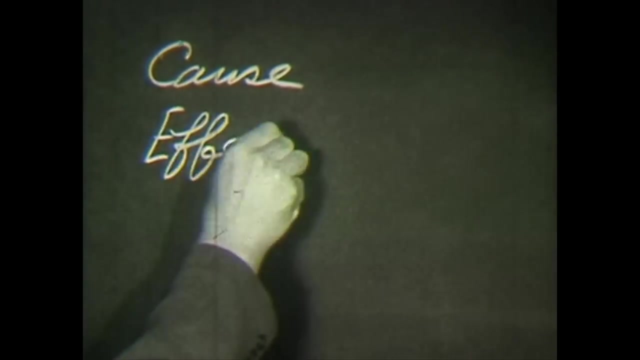 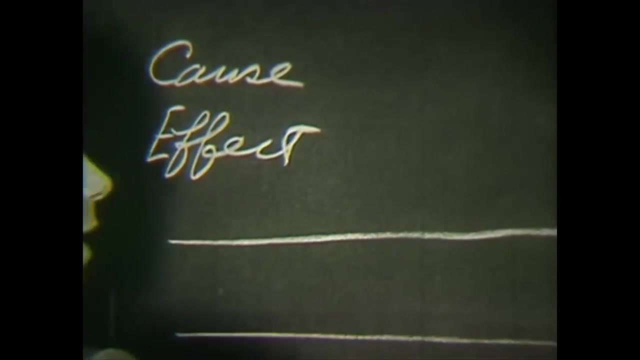 medium. The generation of waves on a transmission line of any kind- electrical, optical or what have you- involves two parameters: An originating cause and a resulting effect. In an electrical transmission line, for example, the cause of the waves is an AC voltage applied to the input end of the line, while the result is an AC. 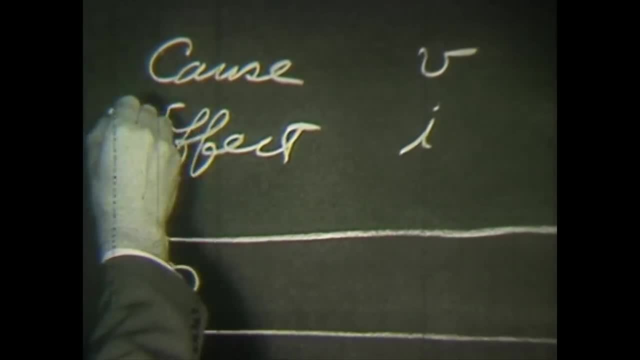 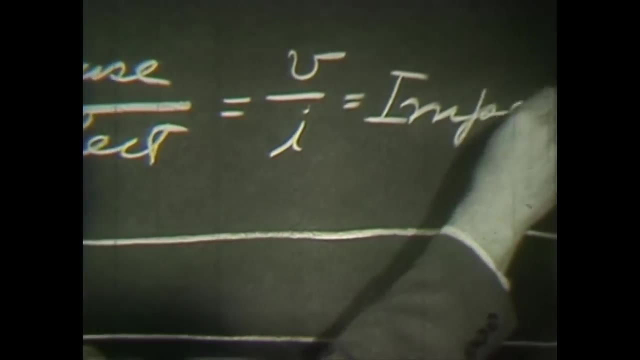 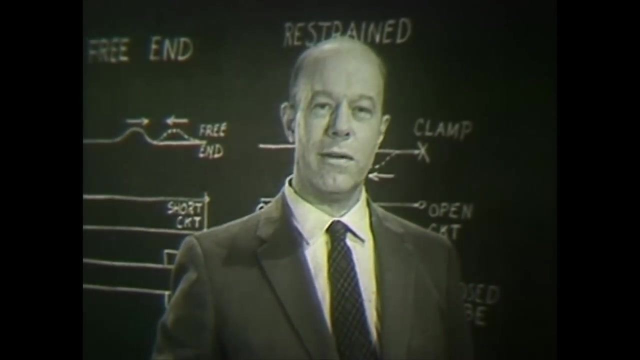 current flowing into the line. The ratio of the cause to the effect is called the impedance. You're probably most familiar with the term impedance through your studies in the field of electricity, but this impedance concept is just as applicable to wave systems of other kinds as well, On our mechanical wave machine. there, for instance, the cause of the waves. 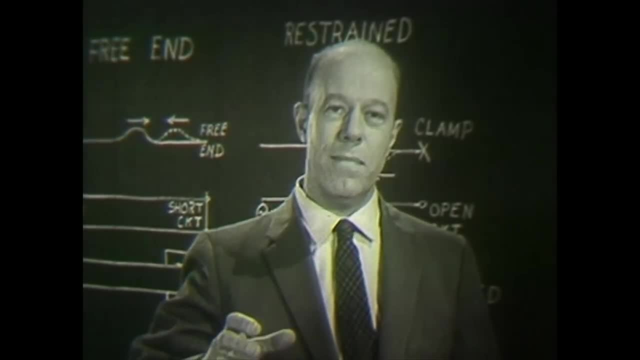 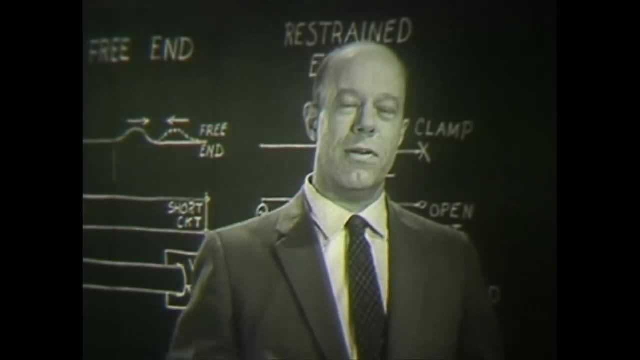 is the oscillating torque which I apply to the first cross arm and the result is the oscillating angular velocity imparted to the medium On that structure. then the impedance- the mechanical impedance- is the ratio of the applied torque to the resulting angular 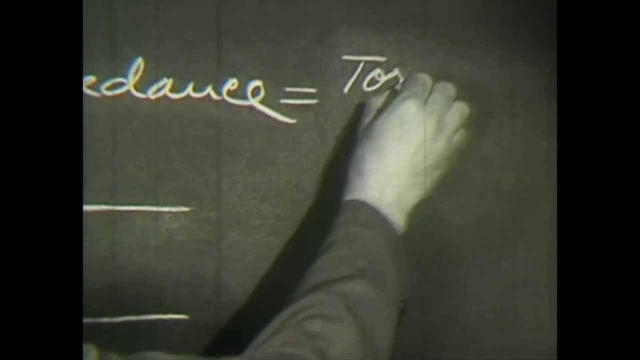 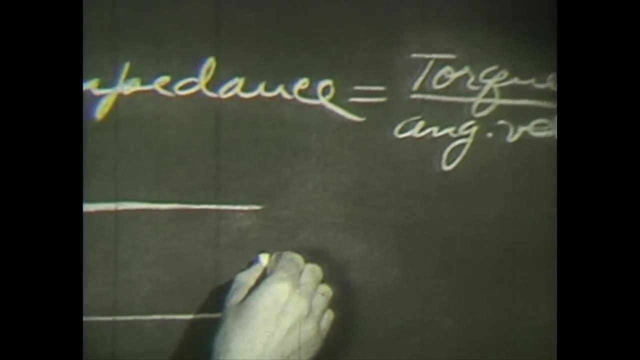 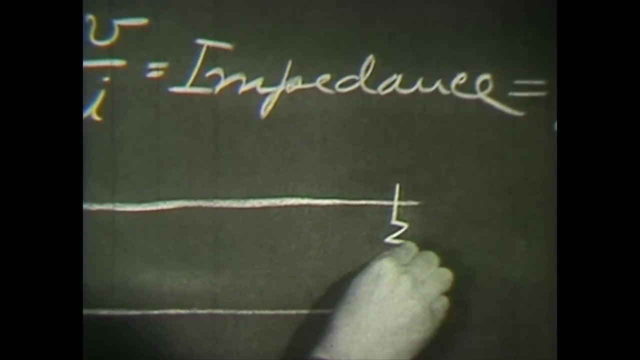 velocity. In terminating the other end of a transmission line, we frequently seek to adjust the impedance of the terminating load to equal the impedance of the line itself. When this is done, all the wave energy traveling down the line is absorbed by the load and no reflection takes. 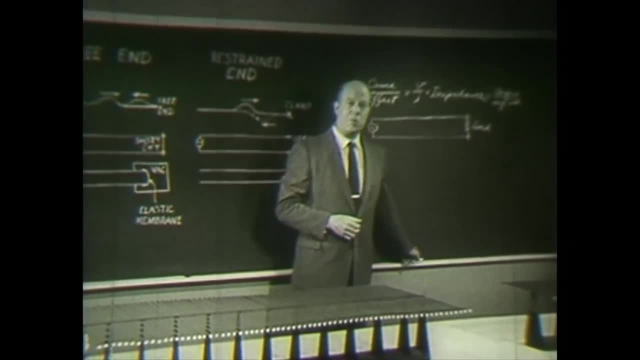 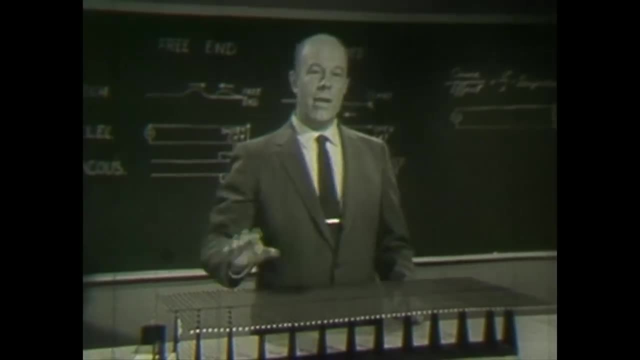 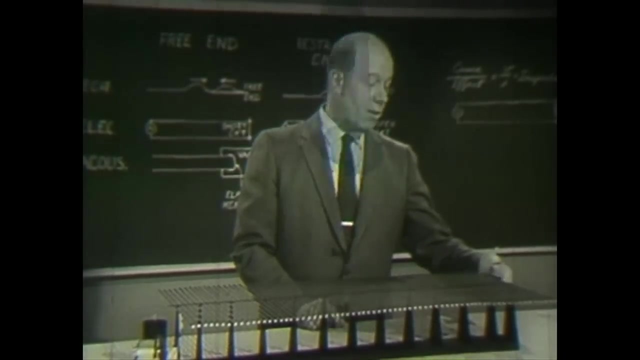 place. The load is then said to be matched to the line. Now this matching condition can be demonstrated very nicely with the wave machine, here by attaching to this last cross arm a mechanical impedance and adjusting the resistance, the counter torque, with which that impedance. 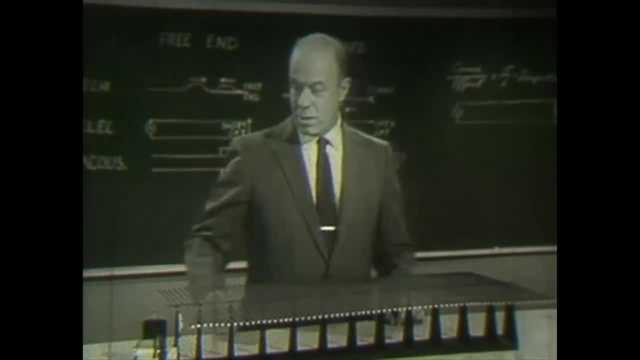 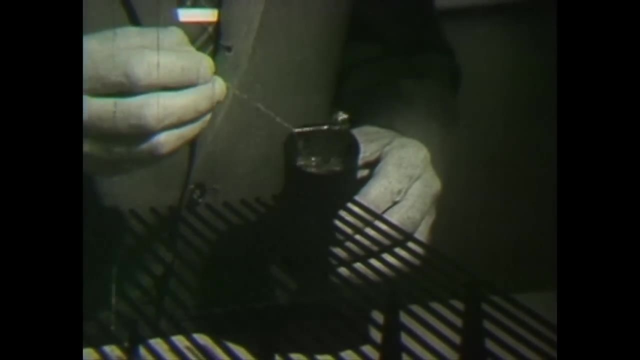 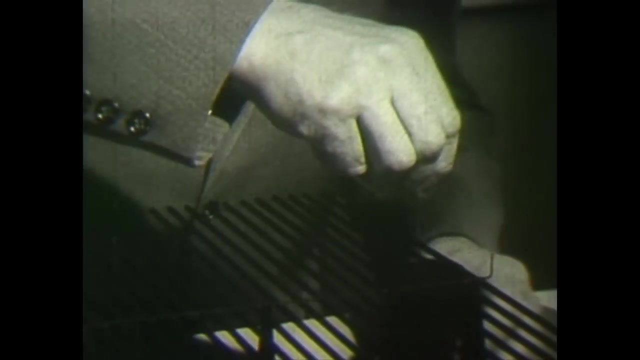 reacts back on the motion of this cross arm. Such a mechanical impedance is afforded by this dashpot, simply a tin can full of water with a little piston pumping up and down in it. By sliding this dashpot in or out along the last cross arm, I can control the counter. 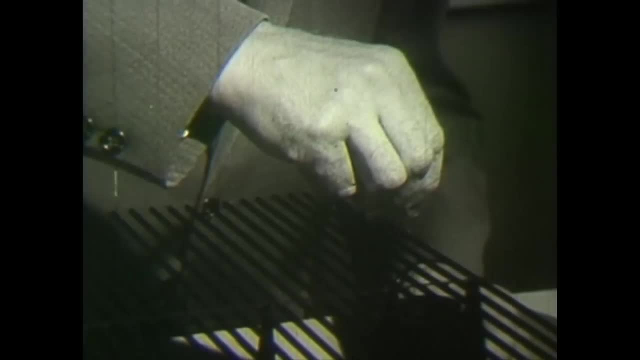 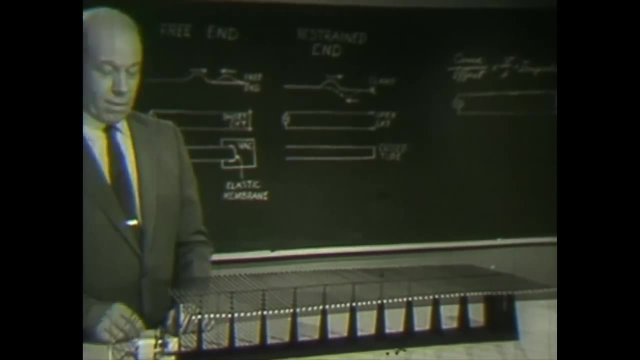 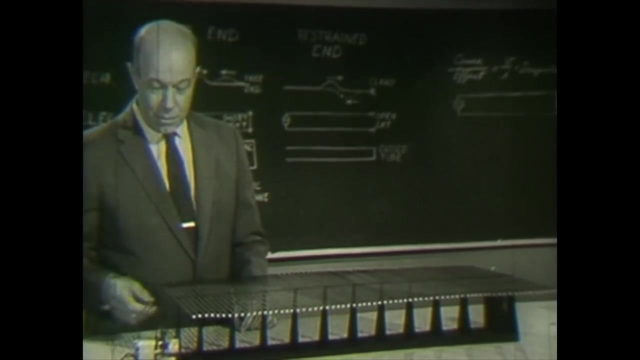 torque with which it resists the displacement of the medium and thus match the impedance of the dashpot to the impedance of the transmission line itself. When this adjustment is properly made, the dashpot absorbs all the wave energy that travels down the line and, as you can, 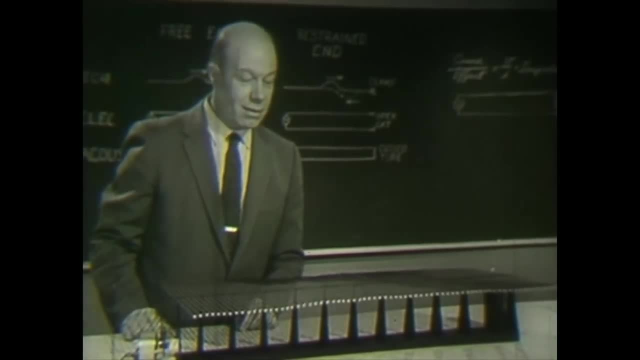 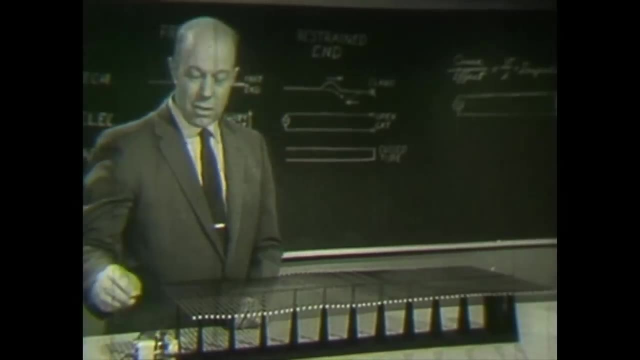 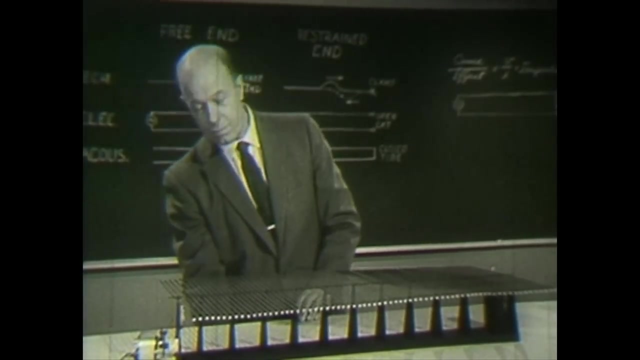 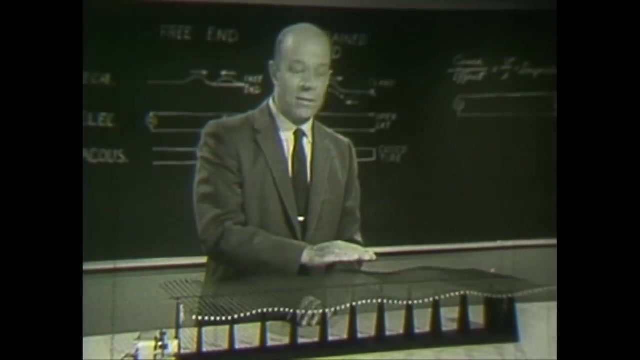 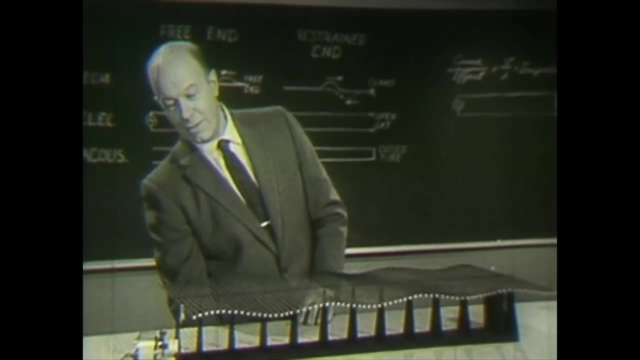 see, hardly any perceptible reflection takes place. Now, instead of using single waves, suppose we have a look at this behavior with a train of continuous waves. Here you see such a train of waves traveling down the machine from the generator to the load and disappearing into the dashpot. 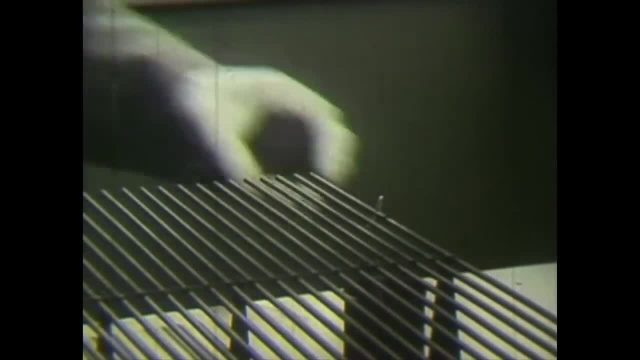 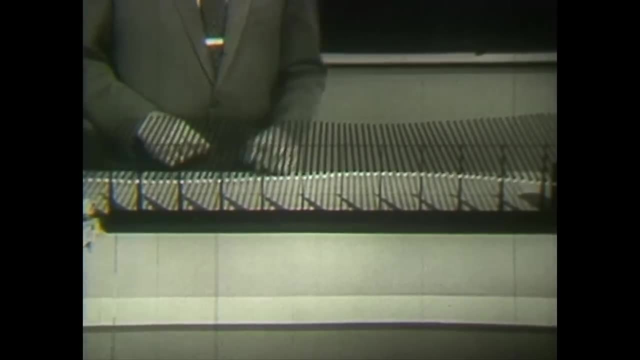 Now suppose I spoil this nice matching adjustment by moving the dashpot farther in toward the central wire. The impedance of the load now no longer matches the impedance of the transmission line and a partial reflection of the wave energy occurs. Let's have a look at this partial 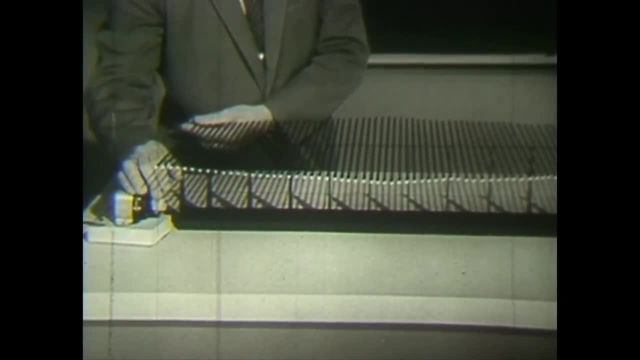 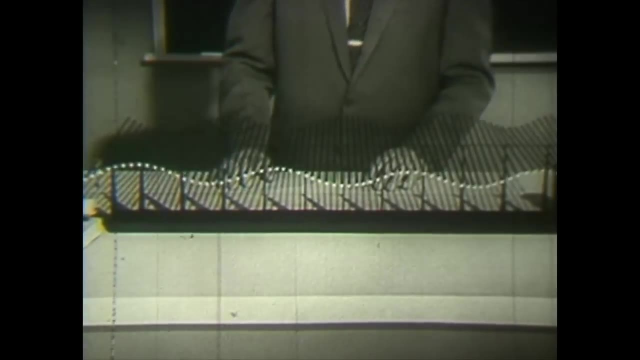 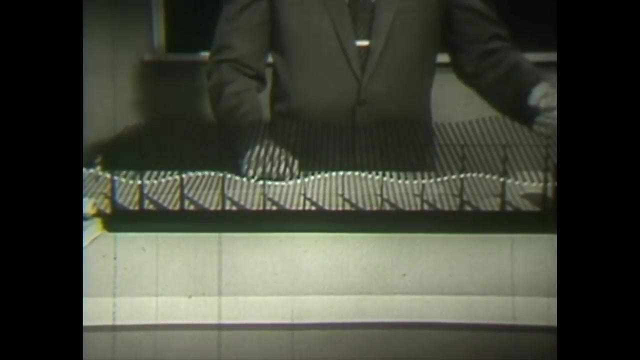 reflection, now with continuous waves. instead, We expect some kind of standing wave pattern to appear on this machine, now, don't we? After all, we have running waves going in this direction and returning waves coming in this direction, of the same period on the same medium, only this time the returning. 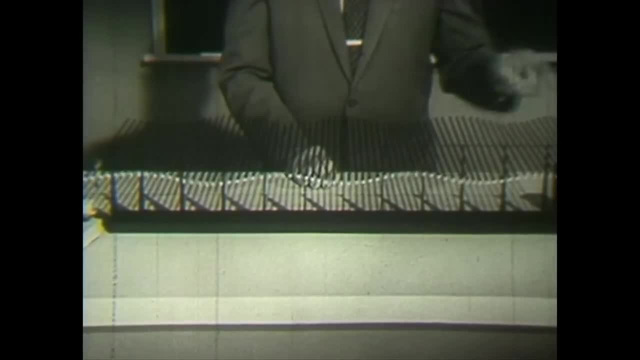 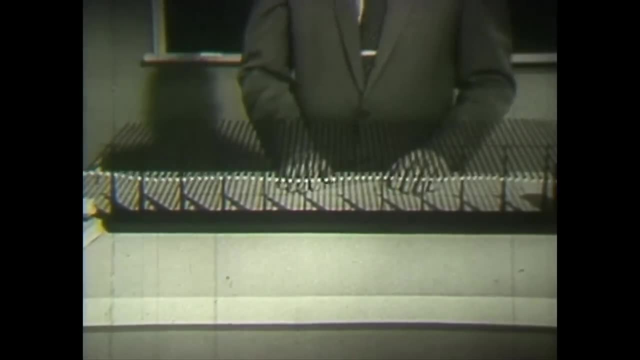 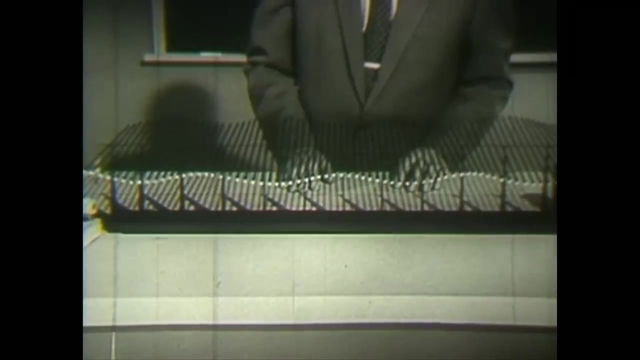 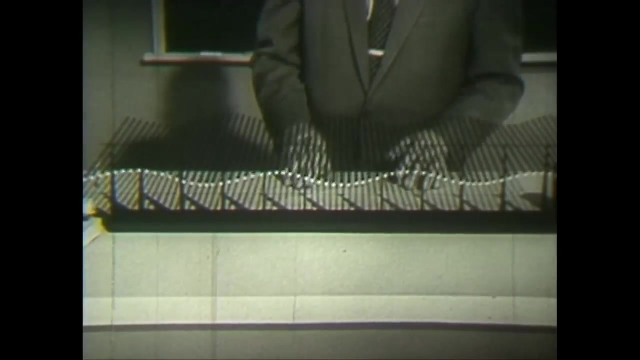 waves have the lesser amplitude because the reflection down here is only partial. Well, I do see a standing wave pattern of sorts. Here are the nodes, nodes half a wavelength apart. Only notice now that the nodes are no longer standing still as they were in the case of 100 percent reflection, Suppose I have the camera speed. 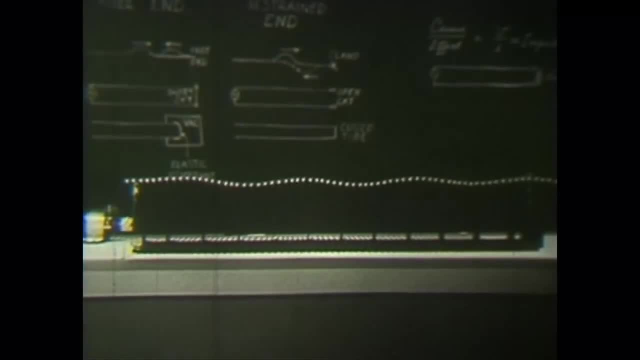 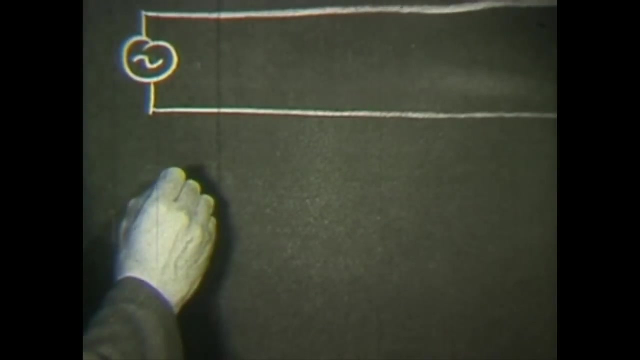 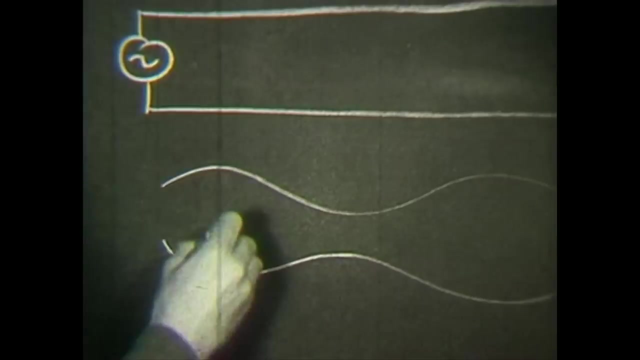 up the picture for you so that you can see what the envelope of this standing wave pattern looks like. Now let me draw you a sketch of that standing wave envelope. The amplitude at this point I'll call sub-maxima, Sub-maxima, Sub-maxima. 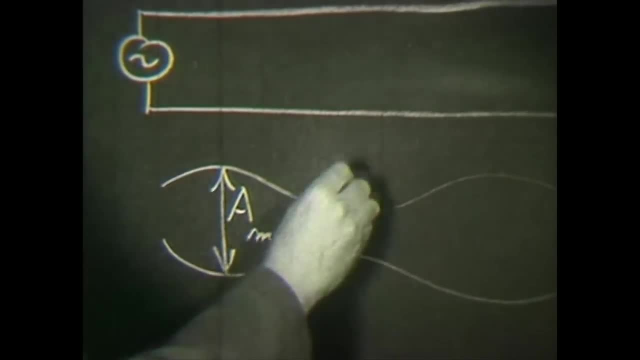 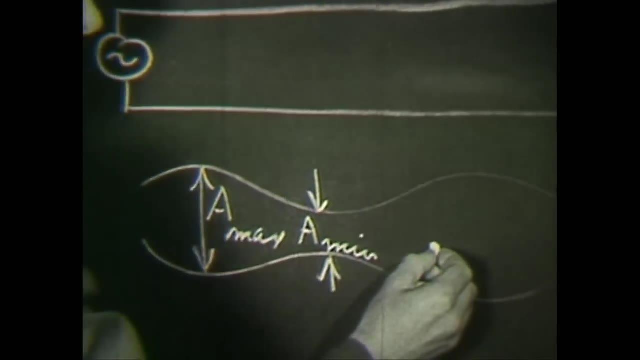 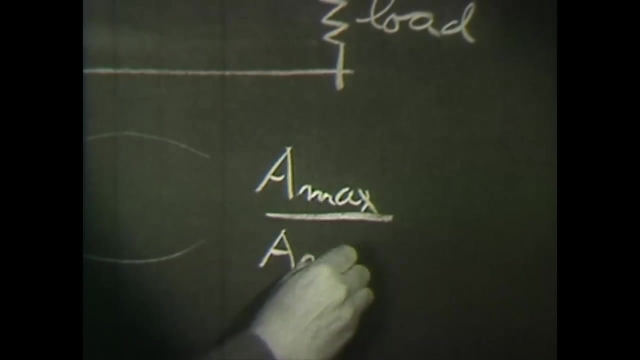 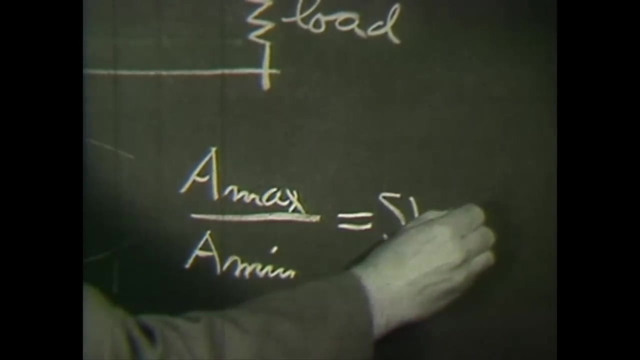 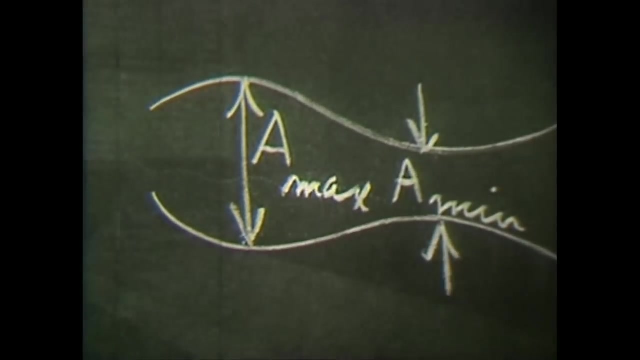 at this point a sub minimum. Now, in wave theory the ratio of a max to a min has a particular significance. It is called the standing wave ratio, abbreviated SWR. On the wave machine, the standing wave ratio is about 3 to 1.. Now recall that when we 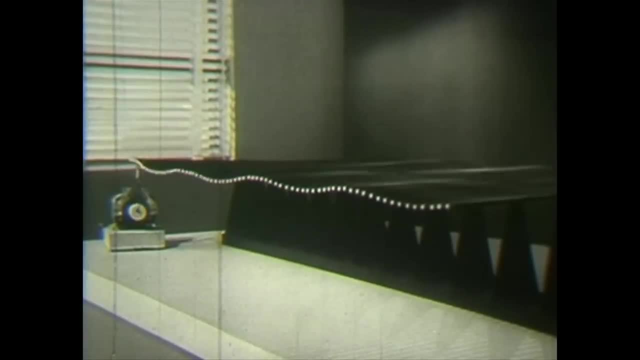 had 100% reflection. when the end of the machine was clamped, we obtained a standing wave pattern with motionless nodes. The standing wave ratio in that case was infinity. On the other hand, when I had a perfect impedance, match there. 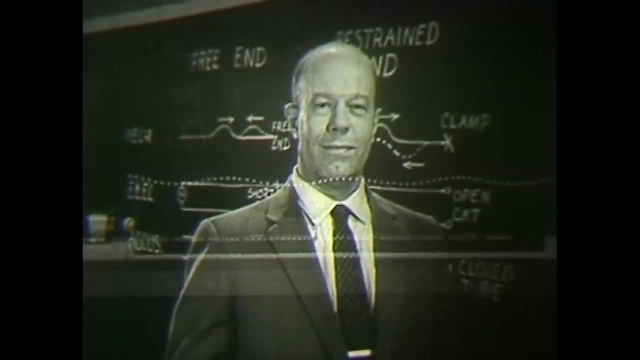 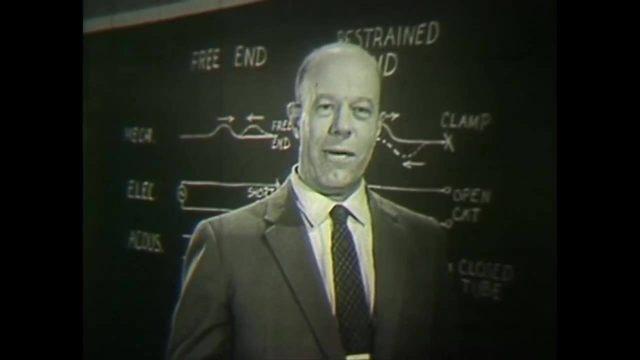 was no reflection at all and no standing wave pattern. In that case, a max and a min were the same and the standing wave ratio was the same. Now I think you can begin to see where I'm leading you. The punchline is this: In any 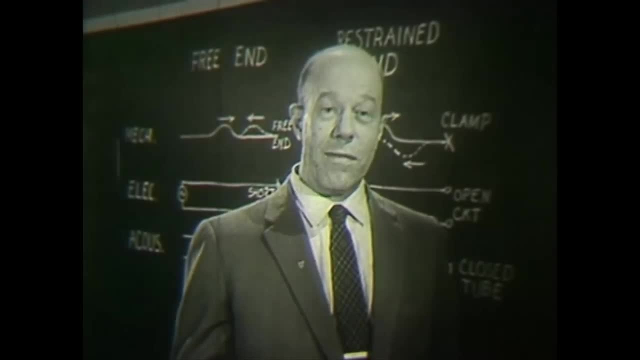 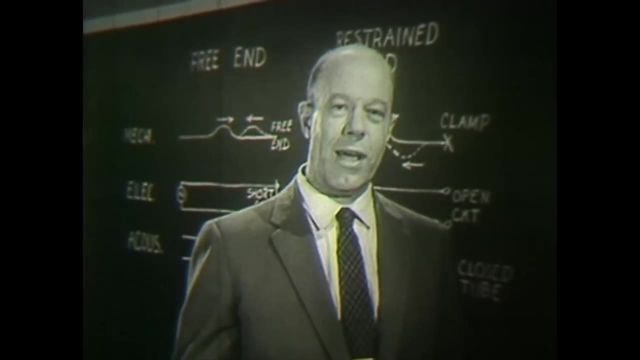 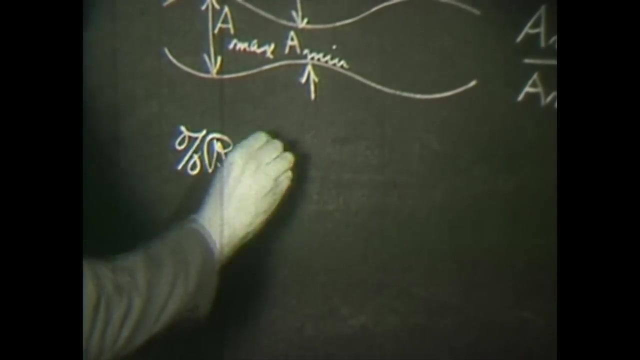 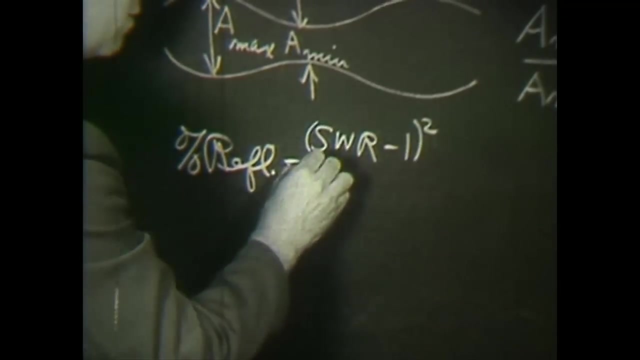 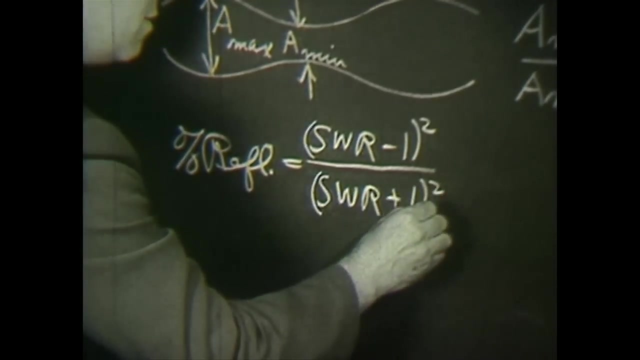 practical case of reflection. a measurement of the standing wave ratio on the medium just ahead of the termination enables one to calculate the percent reflection that is taking place there. The complete expression is: percent reflection is equal to the standing wave ratio minus 1, squared divided by the standing wave ratio plus 1, squared times 100.. 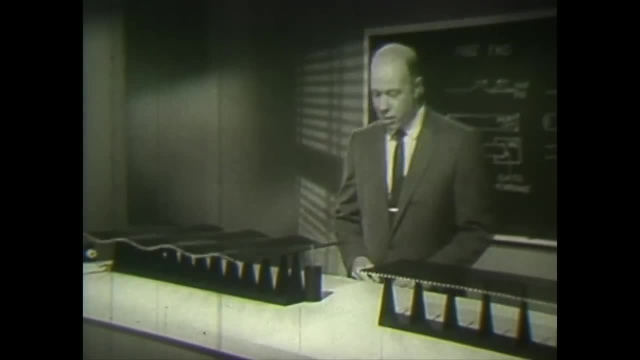 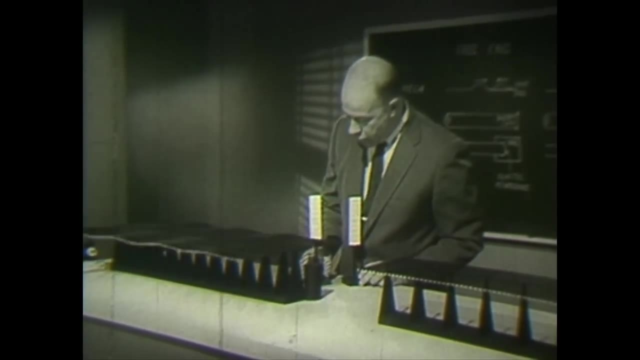 Now, just for fun, let's measure the percent reflection that's taking place here. With these identical scales, I can measure the amplitude at a maximum and at a minimum of this partial standing wave ratio. At this threshold, the amplitude is 1.5. At this, 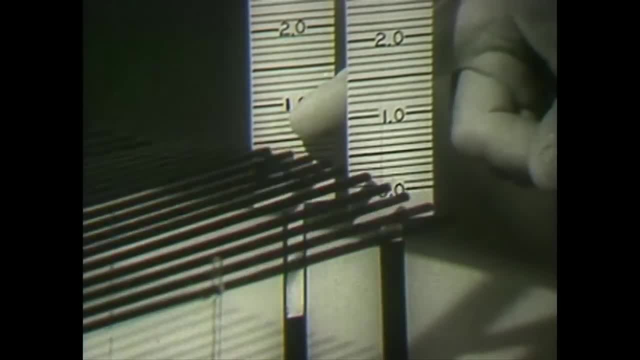 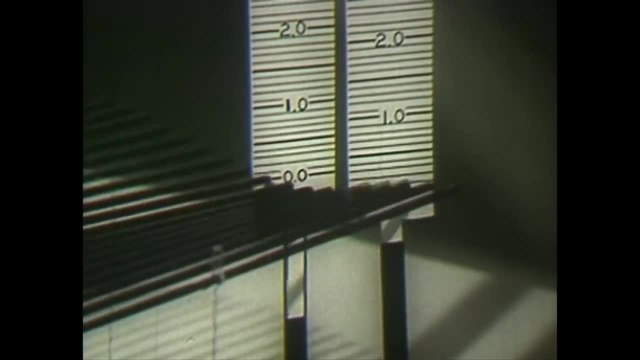 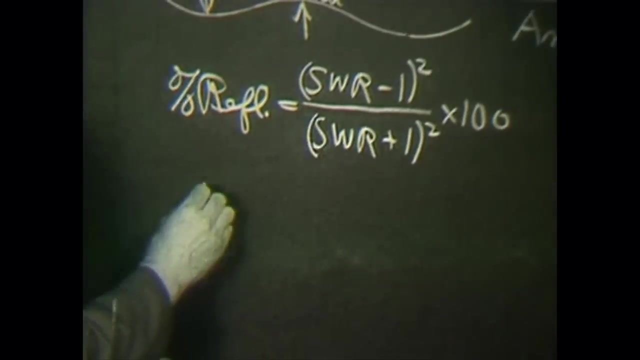 wave pattern: Maximum 5,, minimum 2.. If you and I agree, the maximum amplitude we saw there was 5 units while the minimum amplitude was 2 units. Therefore, the standing wave ratio is 5 halves. Substituting in the percent reflection formula we obtain percent. 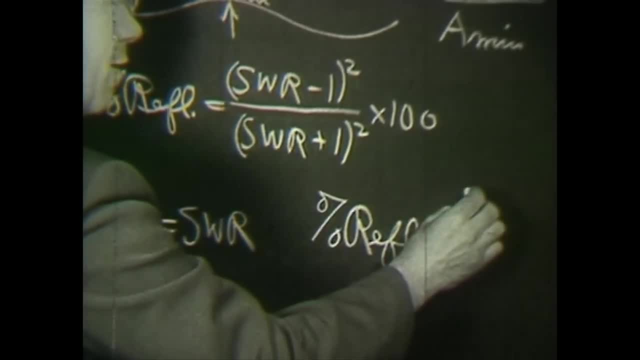 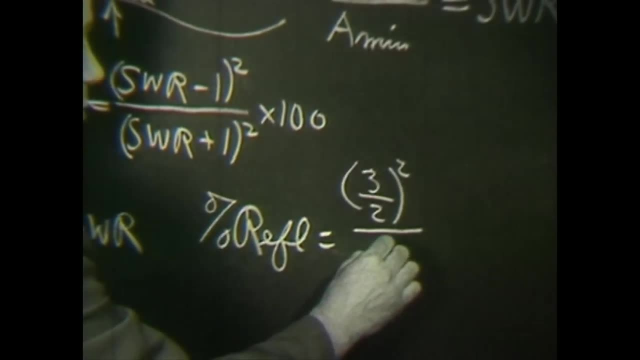 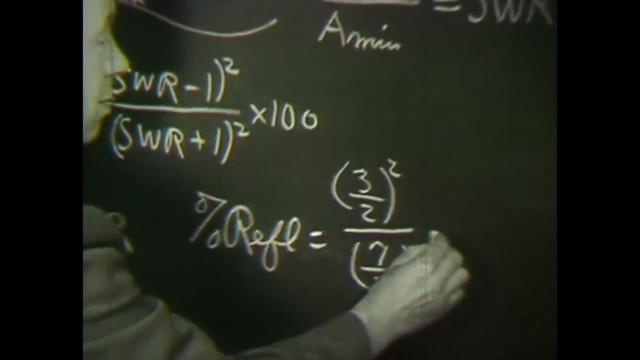 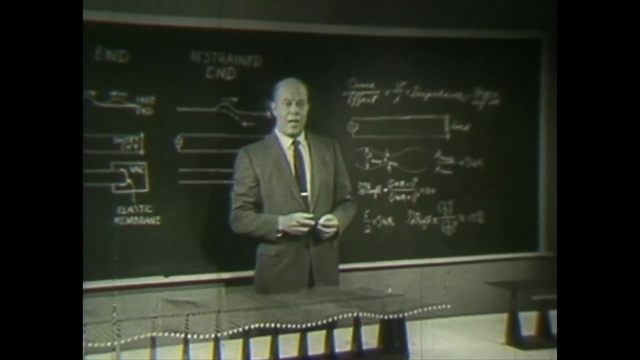 reflection is equal to 5 halves minus 1,, which is 3 halves squared, divided by 5 halves plus 1,, which is 7 halves squared, which gives us 9 forty-ninths or about 18 percent. Now note that I have just calculated the percent reflection on a mechanical wave system using an 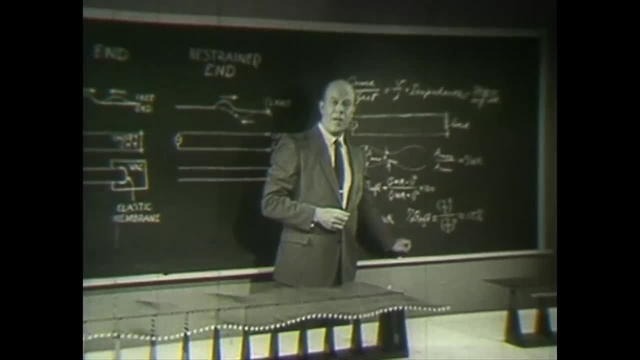 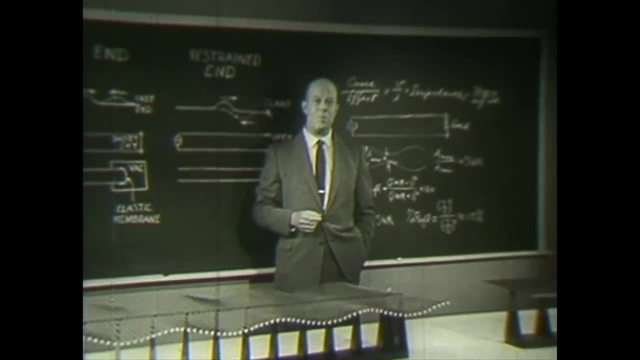 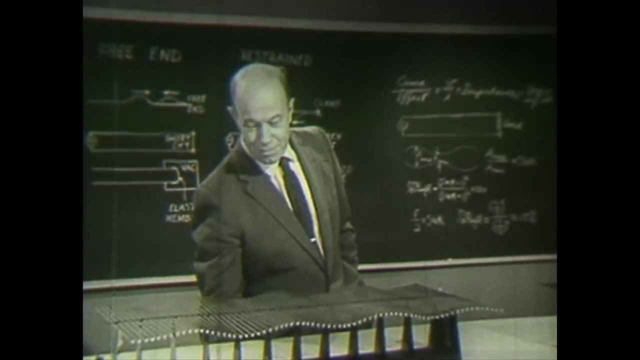 expression that was first developed in the field of AC electricity. Now, this is a perfectly valid and logical thing for me to do, since waves of all kinds behave alike. Now let me develop for you another idea. Waves are partly reflected not only at maximum and maximum, but at maximum and 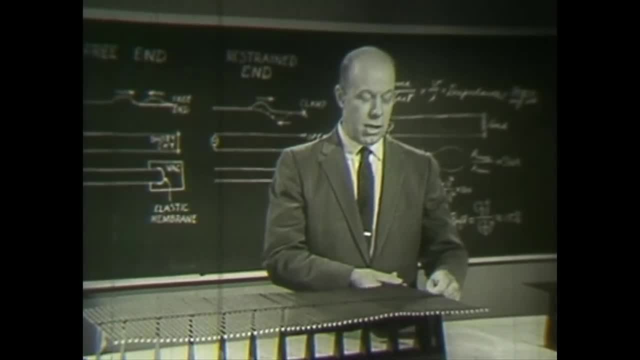 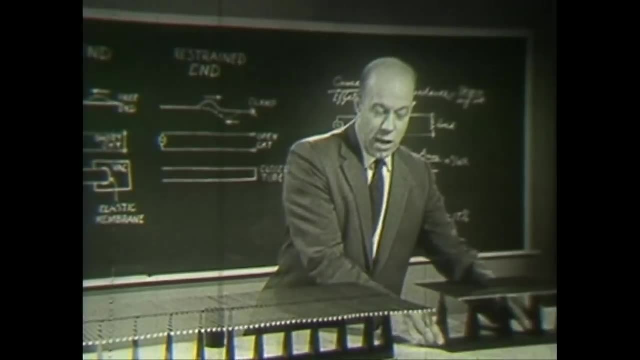 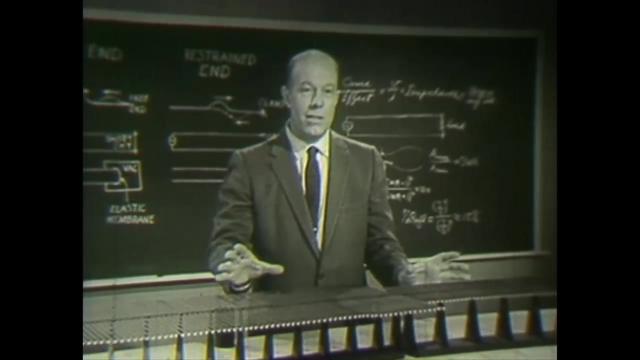 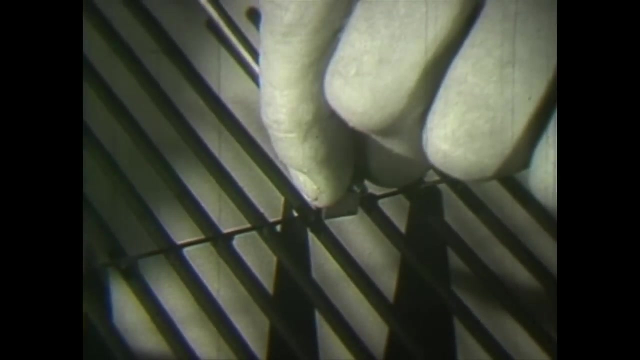 mismatched terminations, but also at places where the impedance of the transmission medium changes abruptly. Suppose I connect these two wave machines end to end Together, they give me a single transmission line made up of two pieces having different impedances. At this point where the two central wires are clamped together with this little clamp, 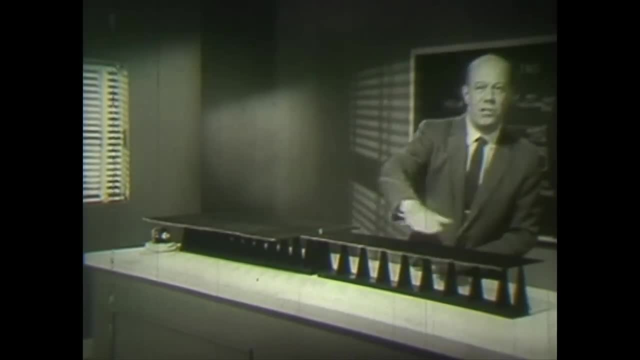 there is an abrupt discontinuity in the impedance of the transmission path. A wave traveling slow along this medium will suddenly speed up when it crosses over into this one. This behavior is similar to what happens to a beam of light when it emerges from glass into air. 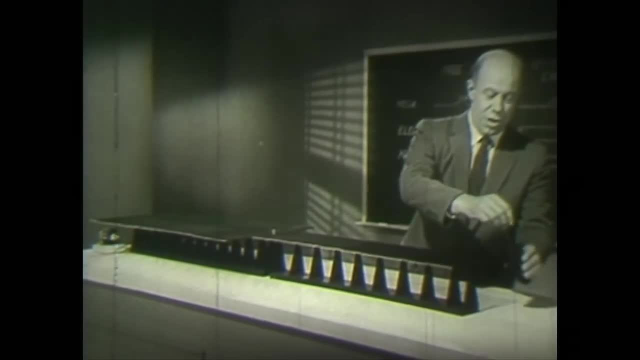 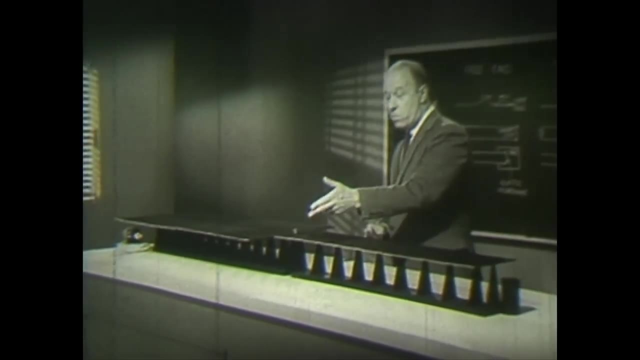 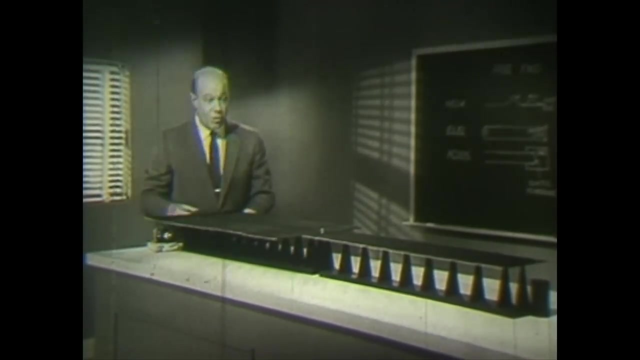 Now, before I show you what I want to show you, let me clip this dashpot down here in a matching position to prevent the unwanted reflections from this end. It's this point. All right, here comes a wave And there it goes Again. Do you see the reflected waves? 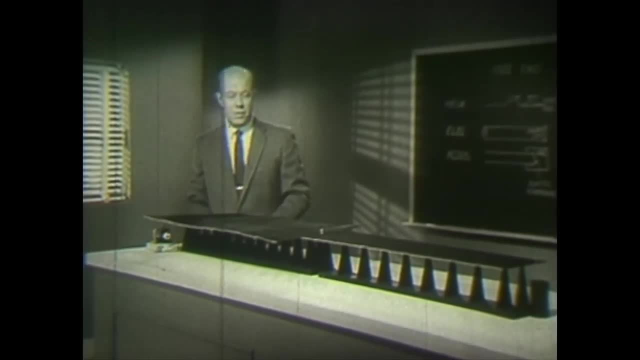 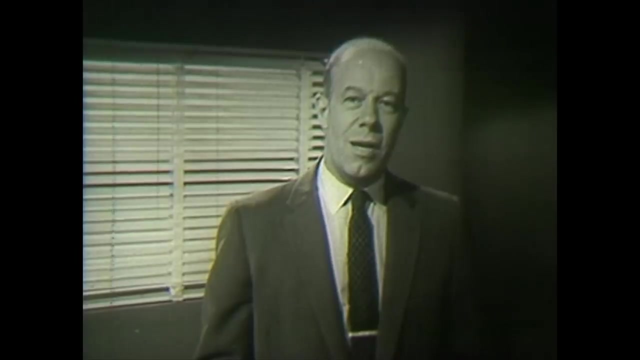 coming back from the midpoint here. Now that I've warned you what to look for this time, you watch for that reflected wave coming back, Here it comes. And once more There goes the main wave, Here comes the partly reflected wave. You know, our world simply abounds in examples of this kind. Electronically. 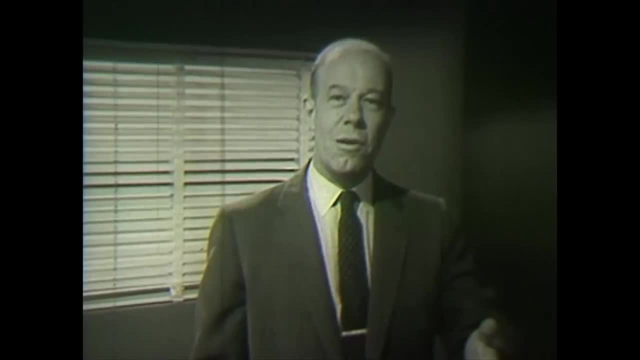 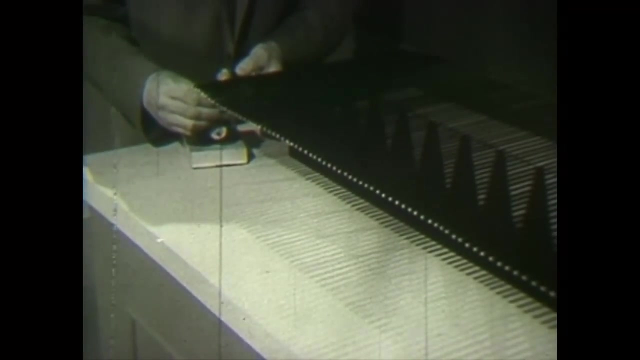 electric waves, light waves, sound waves, mechanical waves, are partly reflected when they encounter impedance discontinuities. Usually in situations of this kind, however, continuous waves are involved. After I connect up this motor, we can see what happens when continuous waves meet an impedance discontinuity, As we might expect, a partial standing wave. 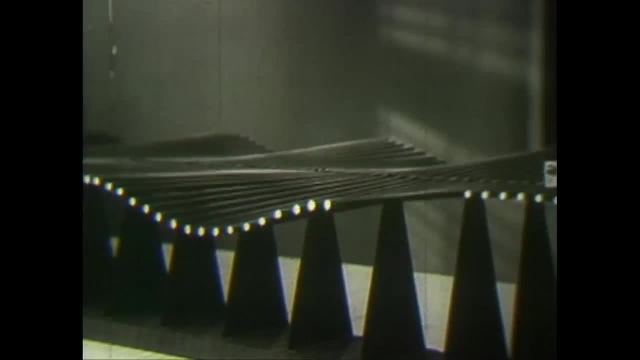 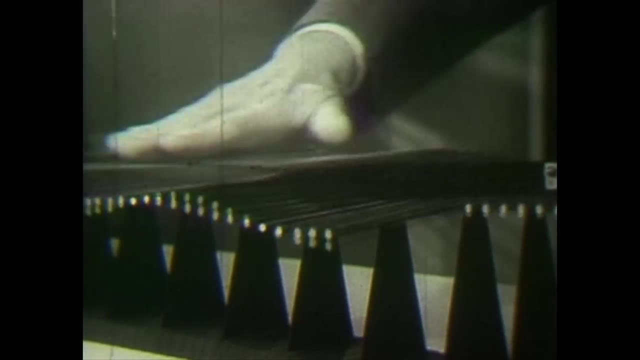 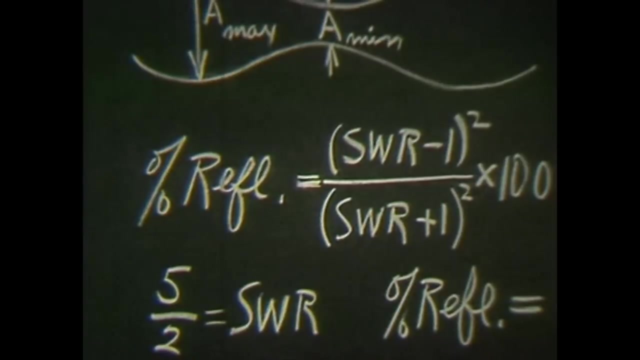 is produced. If I wanted to determine how much energy is reflected there, I could measure the maximum and minimum amplitudes of the envelope and calculate the percent reflection by the standing wave ratio method we used before. That expression is equally good for calculating the energy. 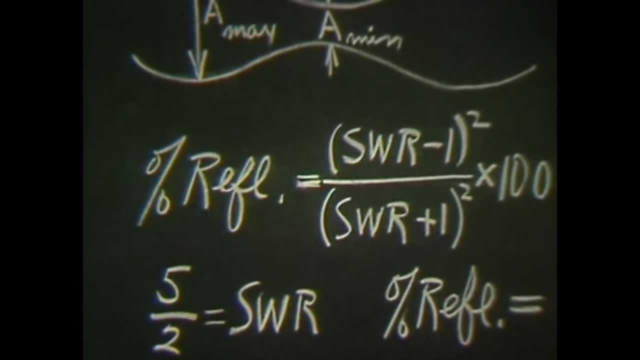 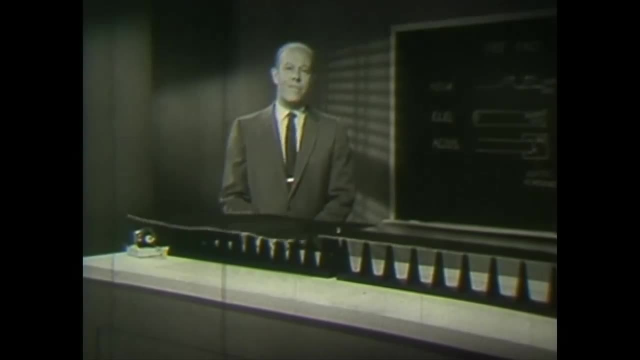 loss at any kind of impedance mismatch or discontinuity. Often in our technology this partial reflection of wave energy by impedance mismatch is considered to be the most effective visual interpretation. The ideal is to generate an скорatio of the wavelength per second. The 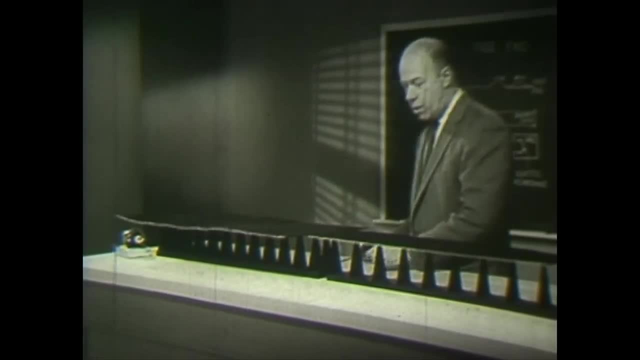 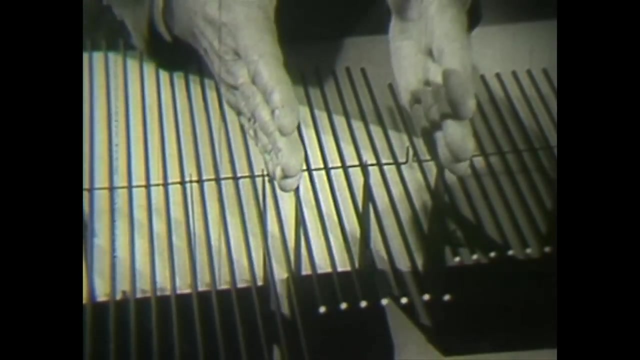 força is very low and in that situation we get an impedence machine in the airway. It's very simple to calculate how much energy each wave has. It is a little more complicated than what we would call a simple paragraph on the. 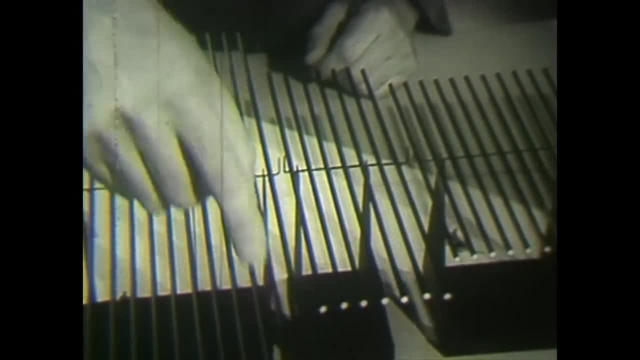 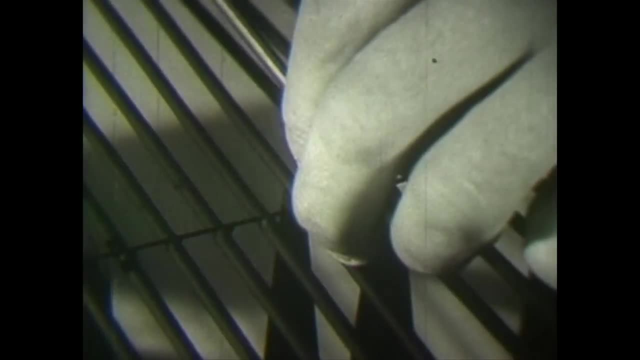 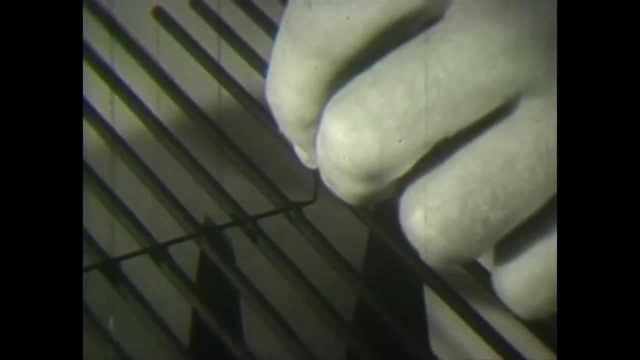 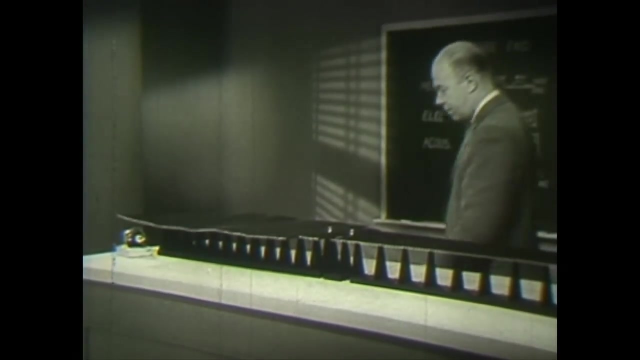 and having a cross arm length intermediate between the cross arm lengths of the two machines. It is called a quarter wave matching transformer. I'll sandwich it in here and then show you how it operates to promote the transmission of wave energy across this discontinuity without reflection loss. All right, here come the waves, and now you watch what happens. 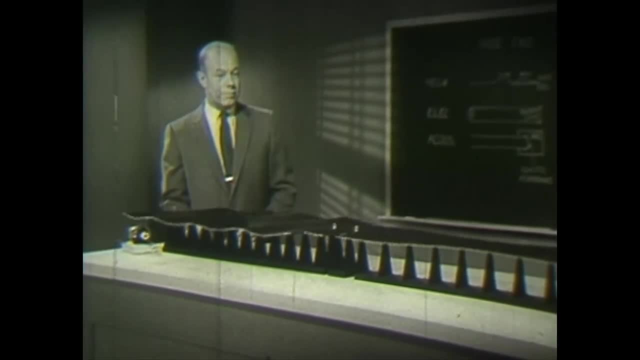 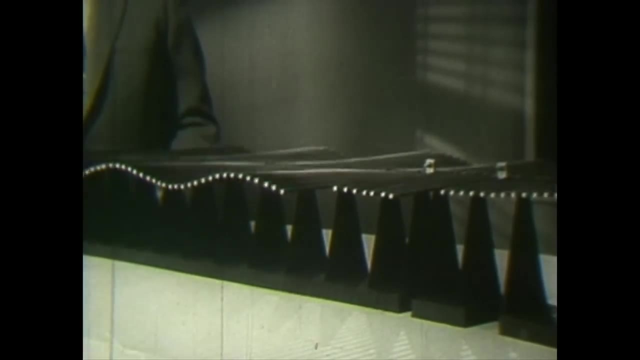 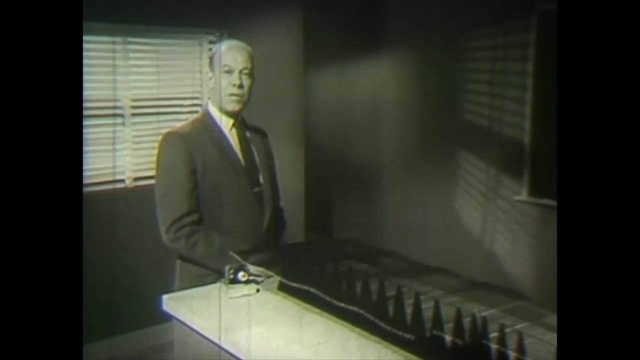 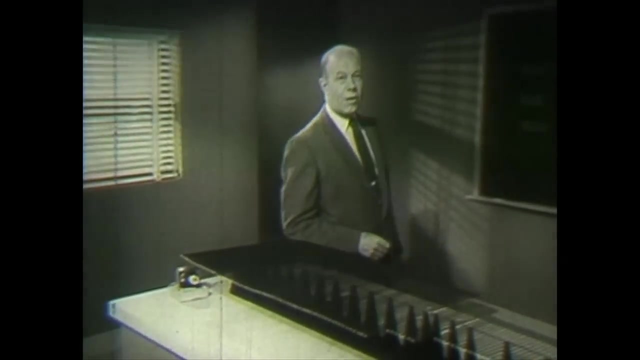 And there they go. There is no perceptible partial standing wave on the input portion of this transmission system, as there would be if reflections were coming back from the junction. Apparently, then, I have matched the impedances of these two machines. This kind of transformer has a direct analog in optics, The non-reflecting coating on the lens of this. 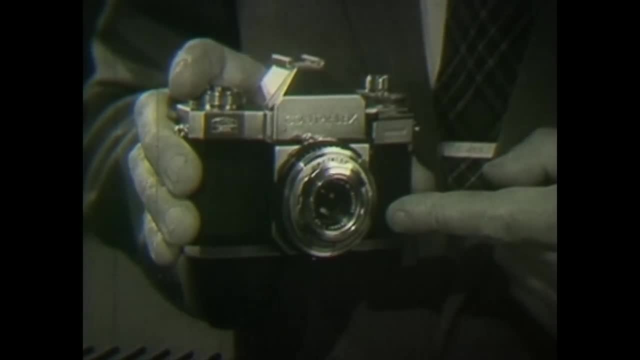 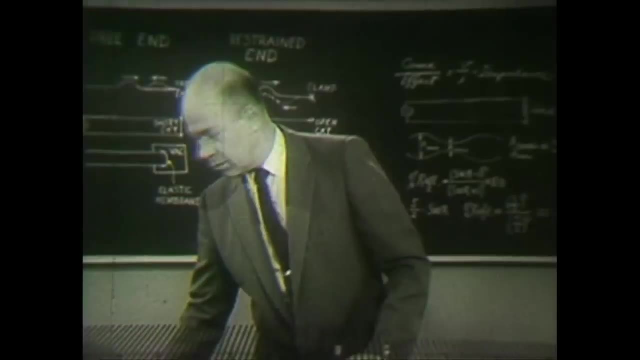 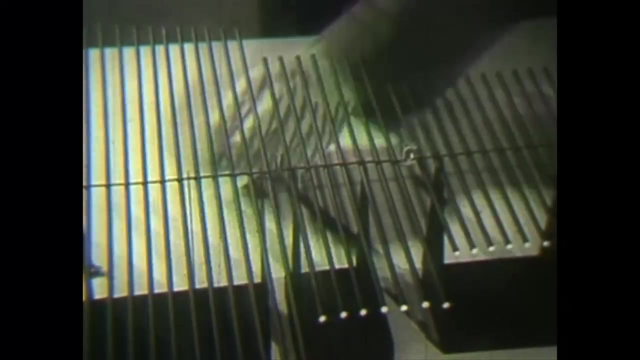 camera is an optical quarter wave matching transformer. It works in precisely the same way with light waves. Now, unfortunately, this type of transformer suffers two major drawbacks: It operates only for continuous waves and it is effective only for a narrow range of frequencies, including the 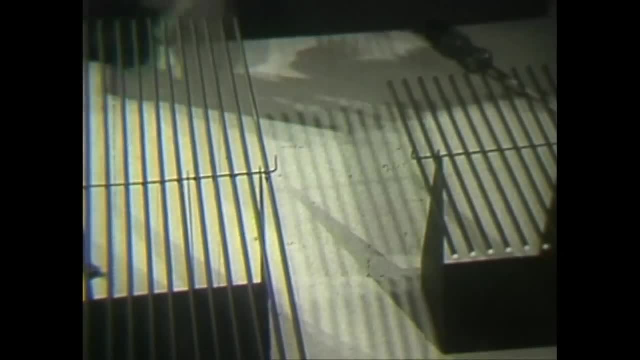 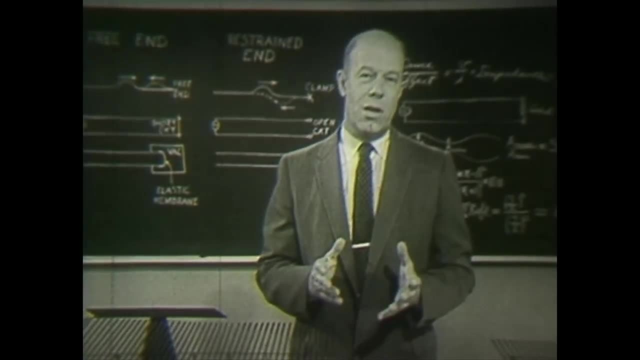 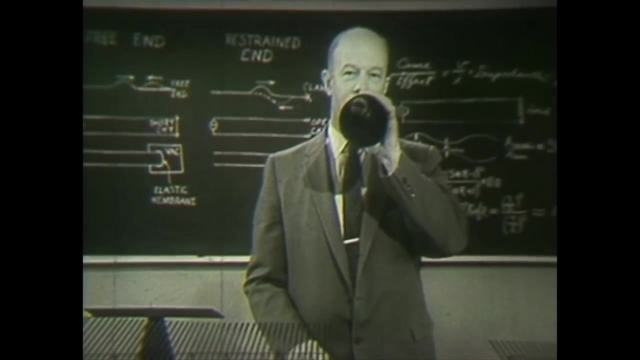 particular one for which it was designed. For applications in acoustics, mechanics, shortwave radio and the like, where it is desired to accommodate much broader ranges of frequency, we have a different kind of matching transformer, to which this megaphone is a first approximation. 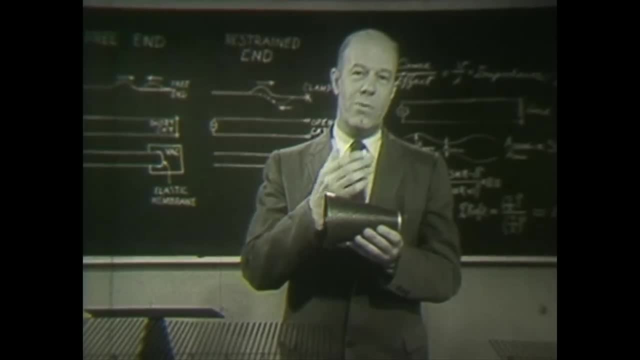 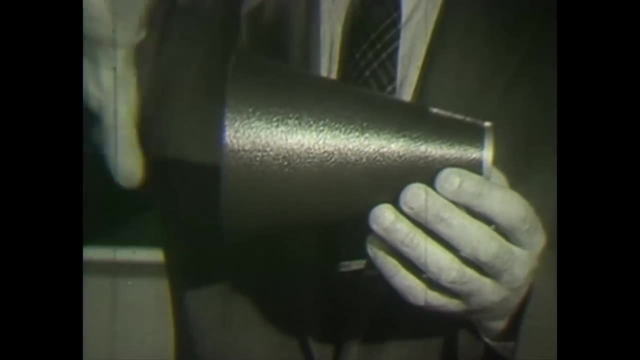 Now the megaphone smooths over the impedance discontinuity between the air column in my throat and mouth and the free air in the space around me by means of a gradual taper. The mechanical analog of a megaphone is a section of the wave medium whose cross arm 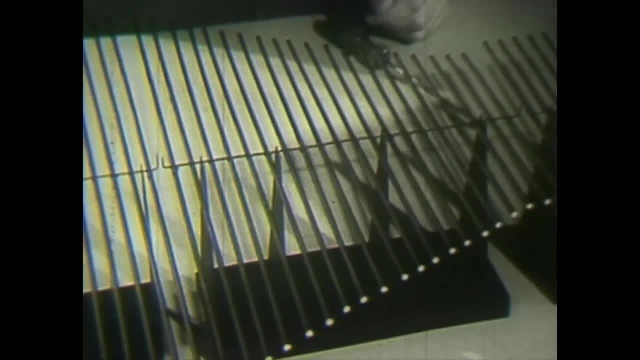 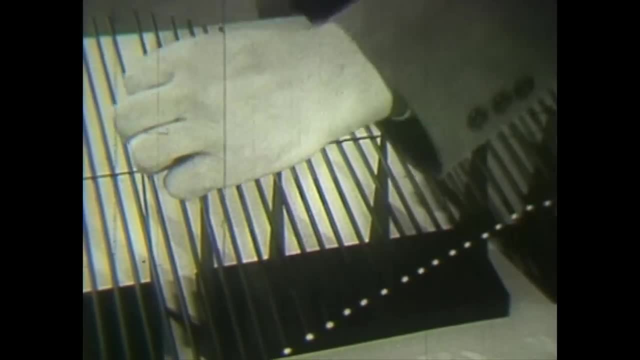 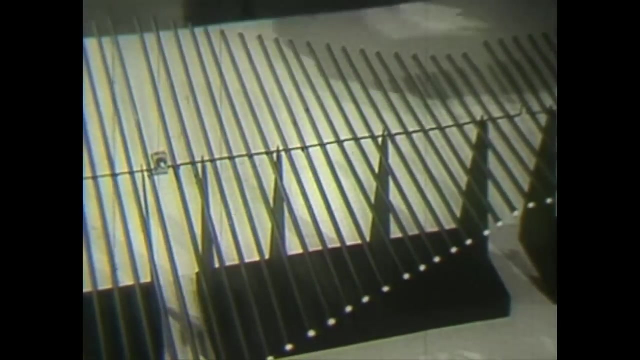 length at the two ends matches the cross arm length of the two machines that I am trying to couple together with a gradual taper in between. A tapered section transformer such as this will match impedances over a relatively wide band of frequencies. It is effective also for use with 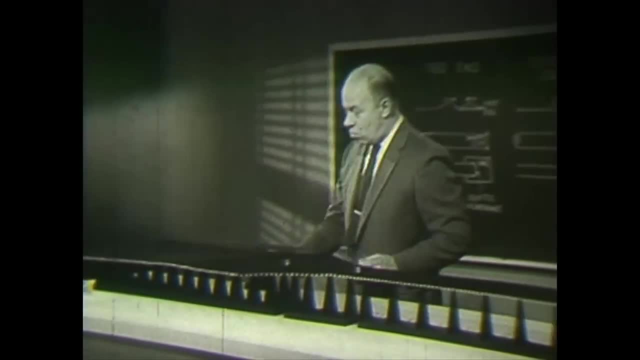 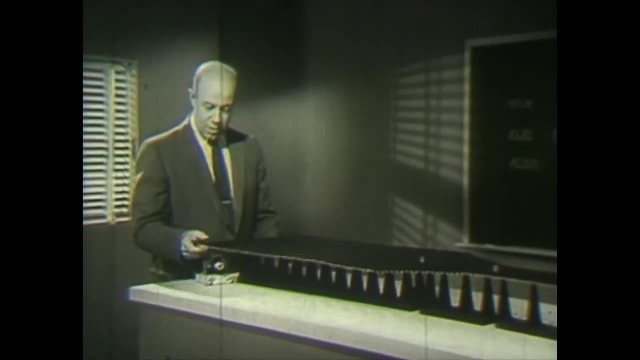 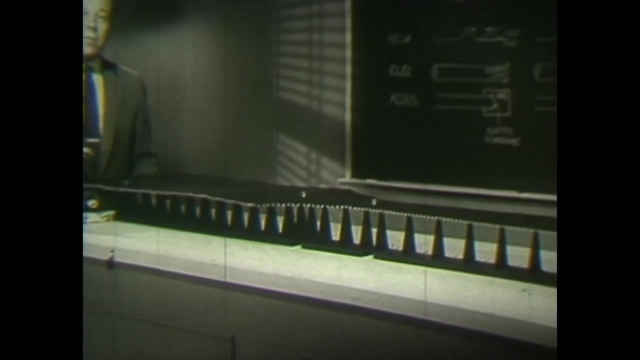 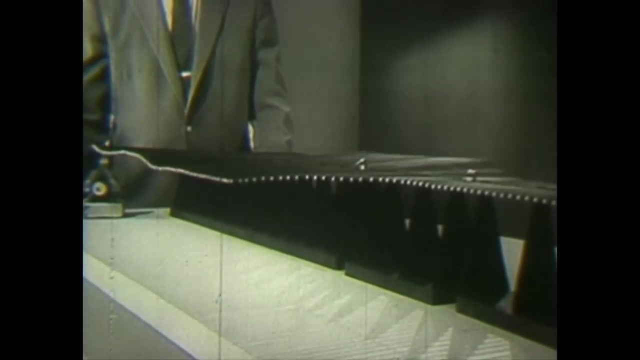 single waves and pulses. Watch what happens now when I send a number of pulses down this line. Here comes a short, quick one, and you see that hardly any perceptible reflection comes back. Here comes a somewhat longer one, and again only a small amount of reflection returns. 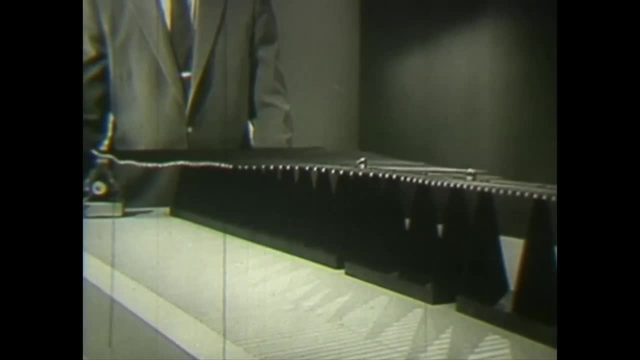 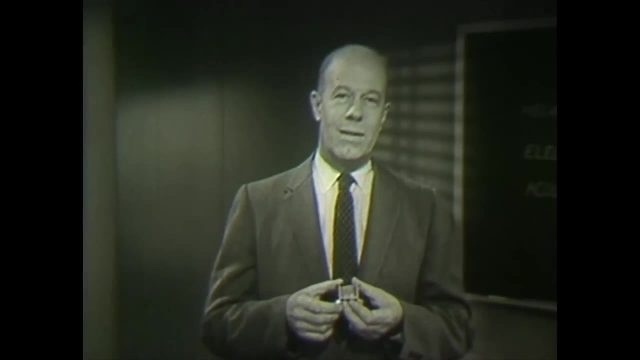 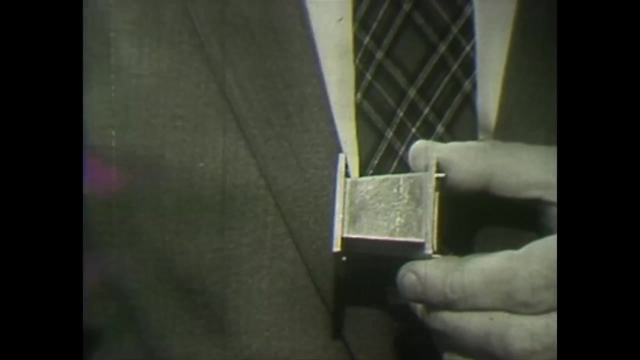 You see, the tapered section transformer is really a relatively broad band device. Here is another example of a tapered section transformer. It is a piece of waveguide. It is used to couple a section of rectangular cross section waveguide to another one of a smaller cross section in such a way as to prevent the reflective loss of radiation. 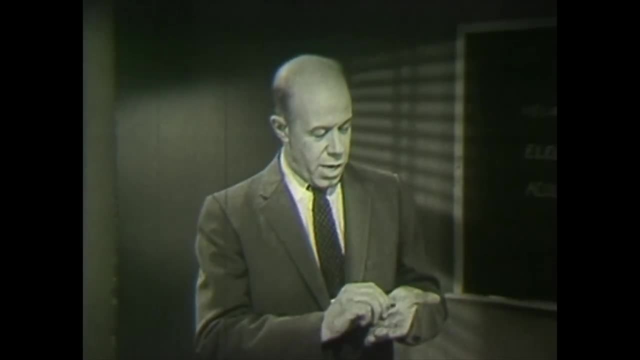 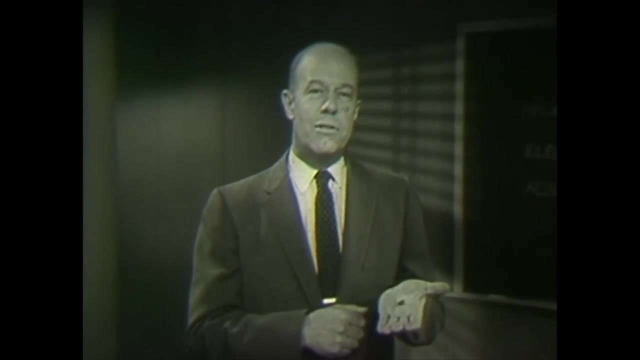 In electricity we employ transformers ranging all the way in size from this little fellow you can scarcely see clear up to the big transformers almost as big as houses that you find in hydroelectric stations. Even nature herself is in their pitching. Inside the mammalian ear there are three tiny bones called the hammer, the anvil and the stirrup. 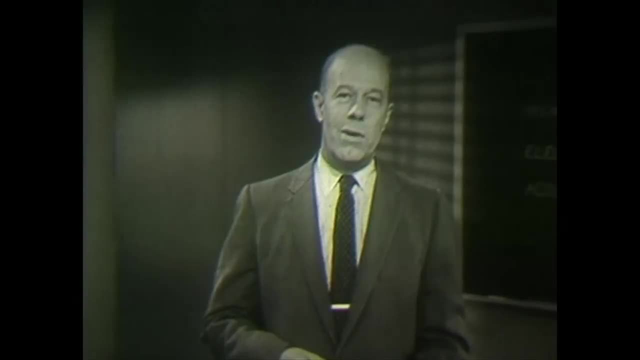 Their task is to provide an impedance linkage between the low impedance of the air in the outer ear and the high impedance of the liquid in the Inner ear. And in addition to all these transforming devices that are used with pulses and waves, there are others that are: 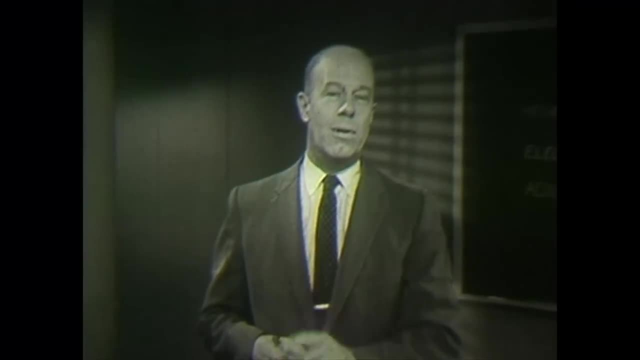 employed with unidirectional motion And should this be done too frequently and every first phase of change costs a lot, Are most heard of near glass surfer's two or three recognize exactly what we call heart refilling of records motion, For example in mechanics, all of the mechanical advantage machines such